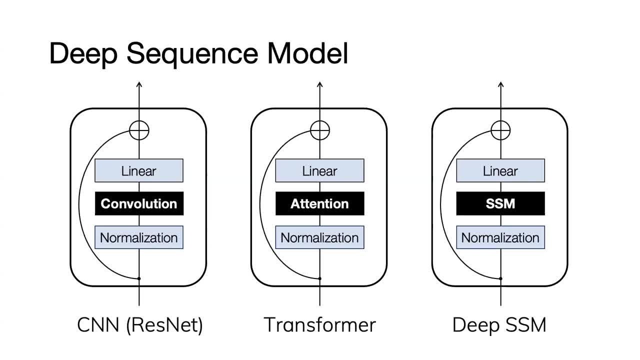 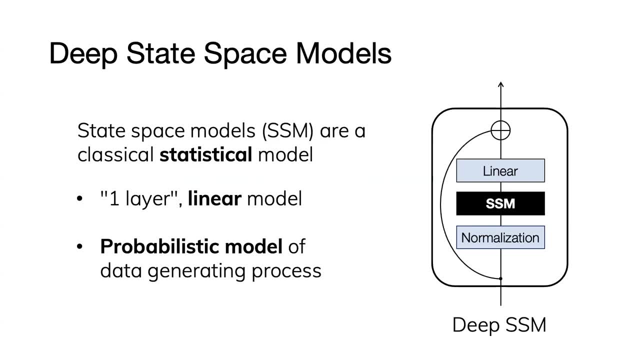 deep neural network in the same way that you would build a transformer or a cnn. so that part is not really our focus. we're going to be looking at what is this in our black box, um to set a little bit more context for people who might know a bit about. 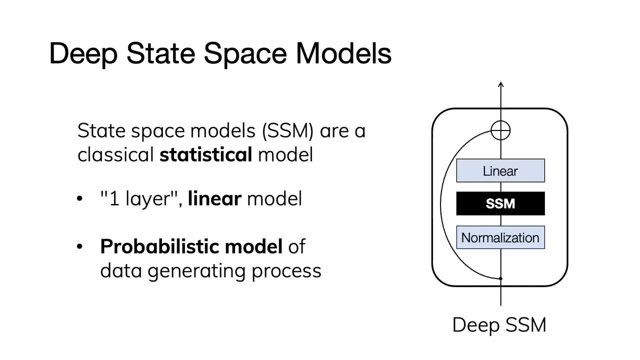 state models- um. they're a really old concept that's been around for a long time. they're usually a statistical model, um, that's been around since the 1960s, um. but in the classical sense they are a probabilistic model where you define, like a, you impose a model on your data distribution and you 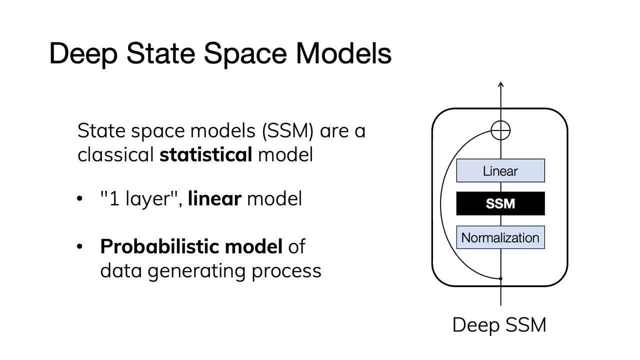 assume your state space model can model that and you kind of have these simple linear models that you can model and you can model that and you kind of have these simple linear models that you can. you can then do statistical inference on, But for us we are thinking of them really in a deep 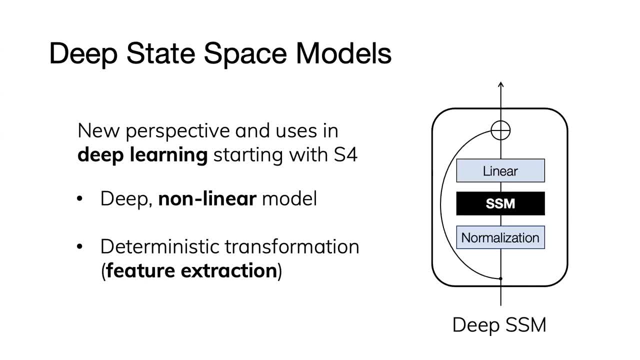 learning sense. And so this is different, because, instead of thinking of it as doing a probabilistic model of the data, the way we think about them is that they're just a deterministic feature transformation, just like you view a convolution as a feature extraction or it's just transforming. 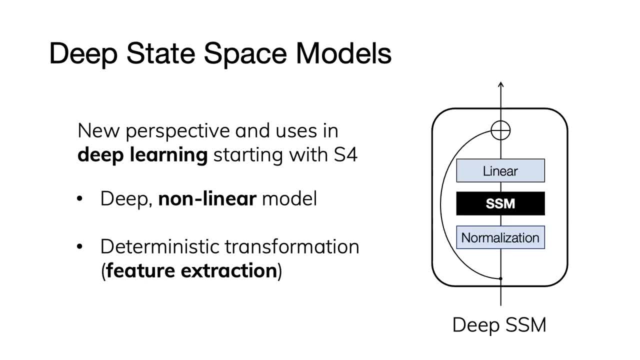 a sequence to another sequence. You're just treating it as a function, And the difficult parts for deep learning are not about statistical inference, but it's about how do you compute these things efficiently? How do you do backprop efficiently? How do you define your model in? 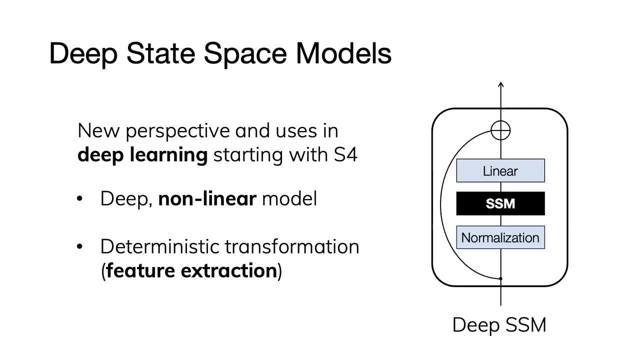 a way that allows it to be extracting meaningful features. So they're called state-based models, but they are a different flavor than what appeared previously, And the model that kind of started this line is the one called S4, which is what this talk is about. Okay, so 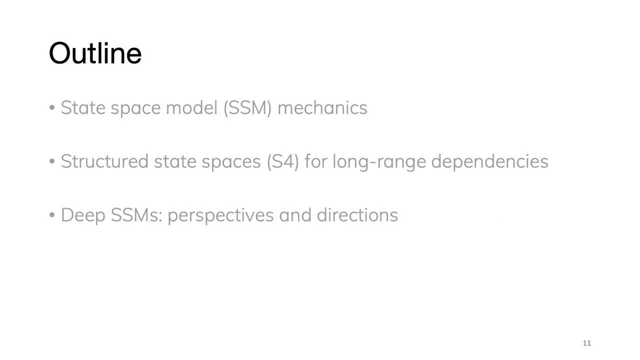 I'm going to show you a little bit of the model. So I'm going to show you a little bit of the model. I'll say how much of this I can get through, but the first two parts of this talk. I'll first talk about these SSMs, or what I call deep SSMs, and how they kind of operate in deep 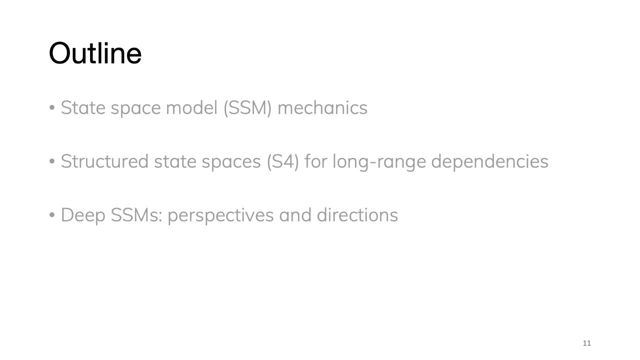 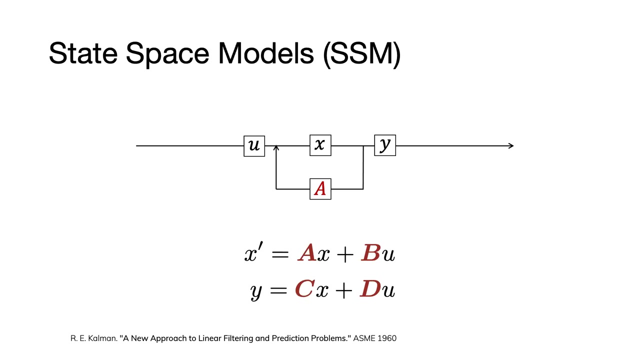 learning and why they're nice in some of their properties, And then I'll talk a little bit more about how S4 relates to these more general SSMs and its special properties. So for this first part, let's just talk about what a state-based model is. This model is a really. it's actually a really. 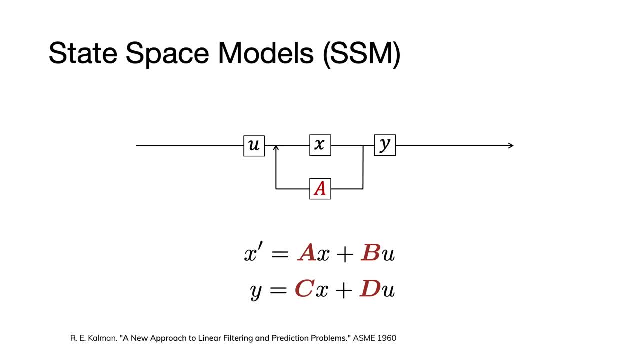 simple model. It's a really simple model. It's a really simple model. It's a really simple model That's defined by these two equations. So here I'll unpack this a little bit more in one second. but basically it's defined through a differential equation And this overall creates a map from this. 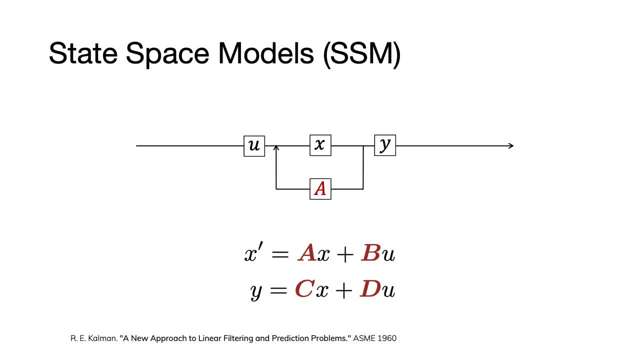 function u. So here all these variables are functions of time. u is a function of time, And then by passing it through this model you get an output. y, that's also a function. These are actually first appeared in controls, and they're kind of illustrated using this control diagram up. 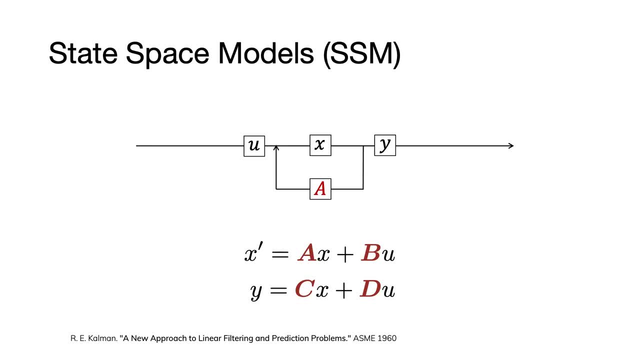 top. S4 is a function of time And then by passing it through this model, you get an output y that's actually a function of 24С, which is not really going to be relevant for our purposes, but just for some context. And, as I said, the first state-based model was the common filter from 1960,. 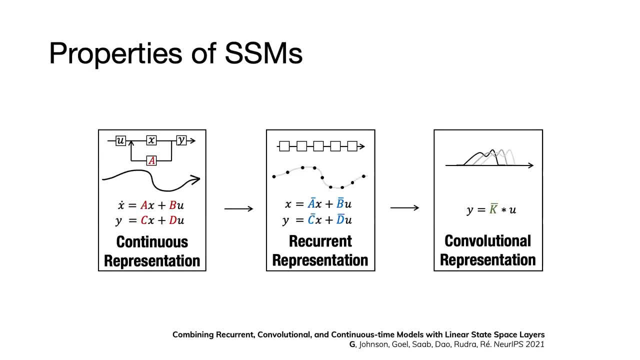 which is still very commonly used Now for us in deep learning. they're going to be nice because they have a bunch of really nice properties for sequence modeling, And so these three properties are going to be that you can view them as continuous models, as recurrent. 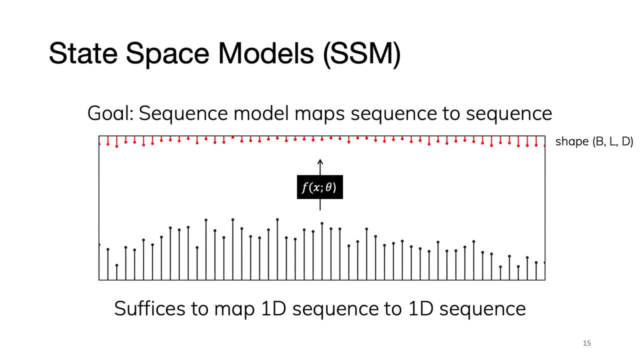 models and as convolutional models, And so we'll go through all of these one by one. Okay, so the first one. So let me just kind of illustrate how this model works as a sequence and sequence map. So again, we were thinking of it as a parametrized function from a sequence. 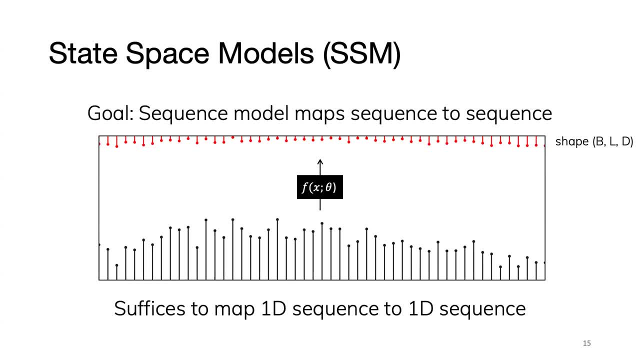 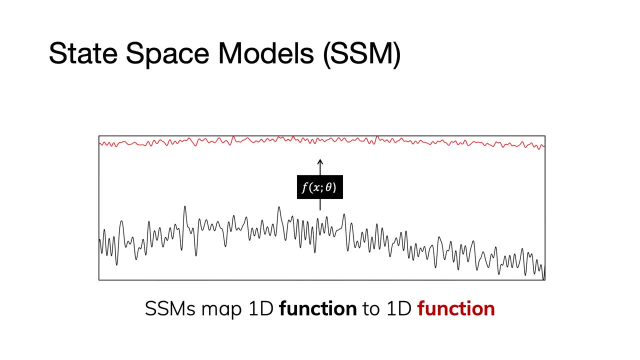 a 1D sequence. a 1D sequence. To be more explicit, the parameters of this function were those A, B, C and D matrices, And then it's going to take an input and give you an output. Now, the way I defined it, remember, is that it's actually a. I defined it through functions. 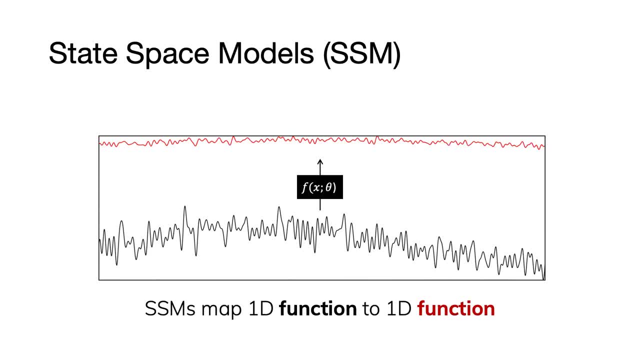 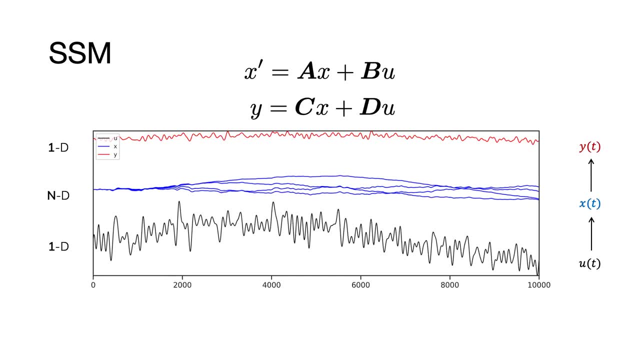 It's a differential equation that operates on continuous functions. So these state-space models actually map functions to functions instead of sequences to sequences, And more explicitly, the way they do that is you can think of, you can just look at each equation one at a 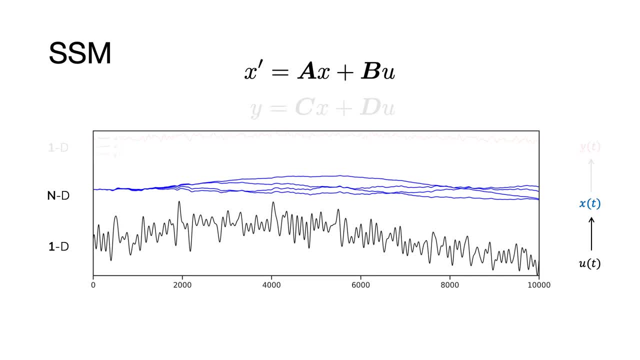 time. So let's look at the first equation. Here at the bottom, this black line is the input function U of T, And now you pass it through this differential equation defined by parameters A and B, And it maps it up to a higher dimensional function. So here, N. 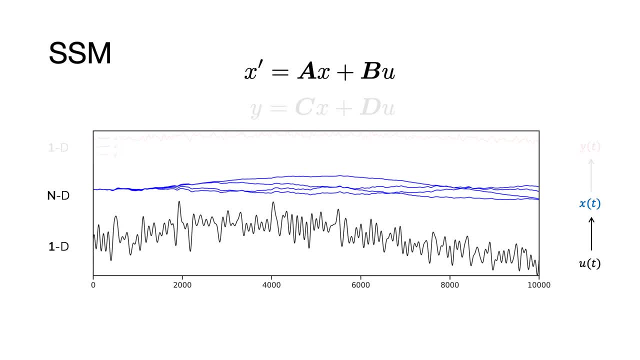 represents the state dimension, which is the order of the intermediate state And this right. so basically, if you just pass this through the differential equation, you get a deterministic output, X, which will be higher dimensional. So, more explicitly, here you think of B as like a column vector, So it blows up the dimension, And then you think of A. 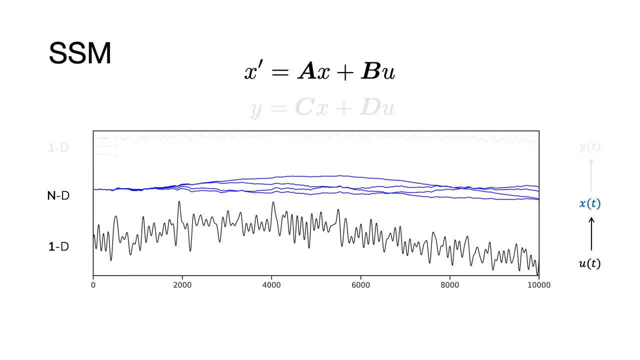 as a N by N square matrix And this is a simple linear differential equation that gives you the state X, which is going to be a vector. So here in blue you can think of like that is, the blue line is X And at any given time X of T. here is a vector of four numbers. 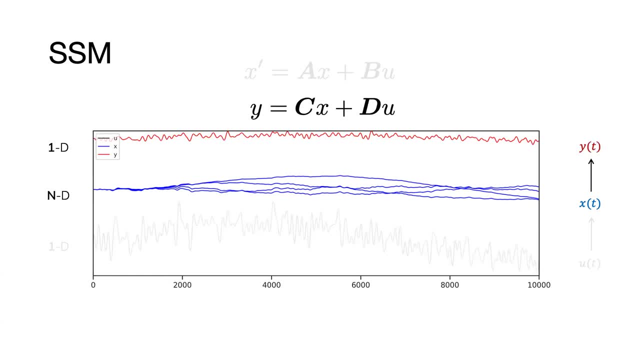 Okay. And then the second equation is much simpler. So this is a map from the state X to the output Y, just by projecting it down back to one dimension. So C here is. you think of it as a row vector that just takes a linear combination of your state features and projects it back out, And that's. 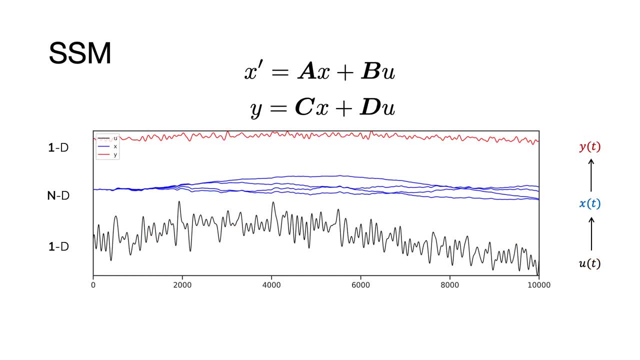 the whole thing. So this is a linear combination of your state features and projects it back out. So this is a linear combination of your state features and projects it back out, And that's the whole definition of what these two equations do. So again, it's a very simple map from a 1D. 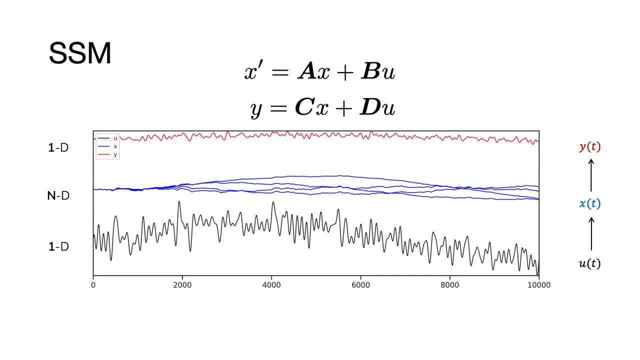 function to 1D function. Yeah, Any questions here, Just like that. That's right. So X is a latent function, U is the input function, X is a latent thing And Y is the output function. And this is just a map from U to Y. That's defining like a. 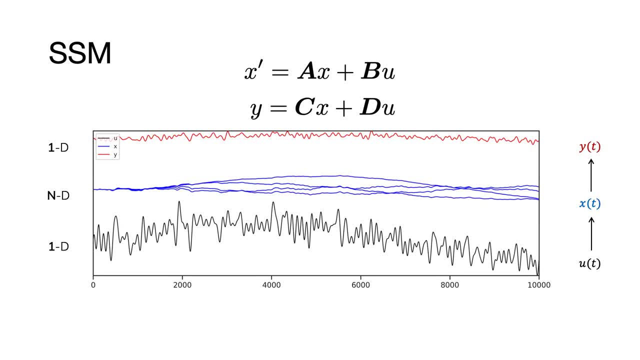 deterministic transformation. Yeah, Actually I kind of regret using this notation. This notation is from controls And originally we're like this for that connection, But it actually confuses people sometimes because, as I mentioned, this is actually quite different from the controls usage. 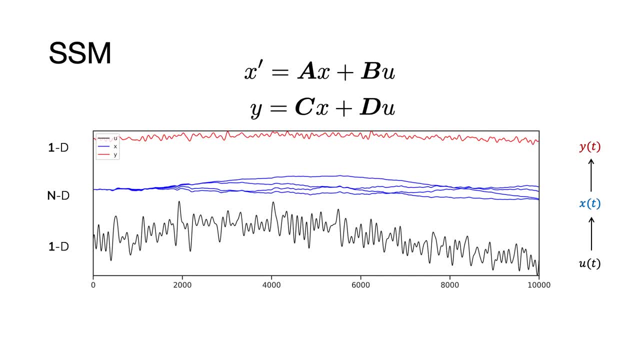 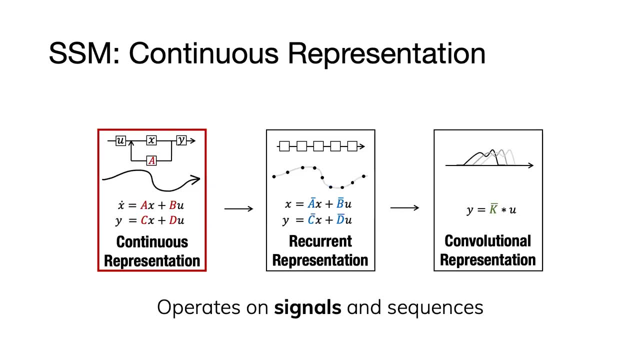 And in deep learning you normally have inputs X, outputs Y And, yeah, at some point I might actually consider redoing the notation, But anyways, Okay. So the first property I mentioned, the continuous representation, is really just saying that. 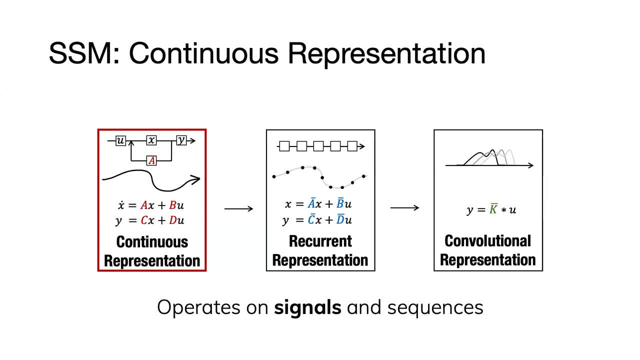 this map operated on functions and not just sequences, So this has some concrete benefits, because functions are in some sense more general than sequences. You can always discretize a function to get back a sequence, And this has some really concrete benefits, such as being: 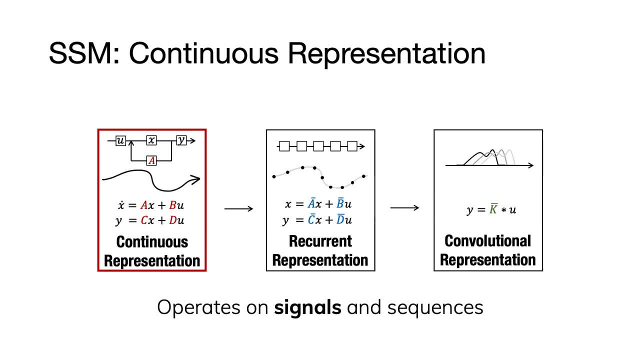 able to operate on irregularly sampled data or stuff like that, where you might want to define an underlying continuous process. Or another example is that some types of data are really based on an underlying function or an underlying signal, such as lots of perception data like images and audio. There's like an underlying audio waveform. 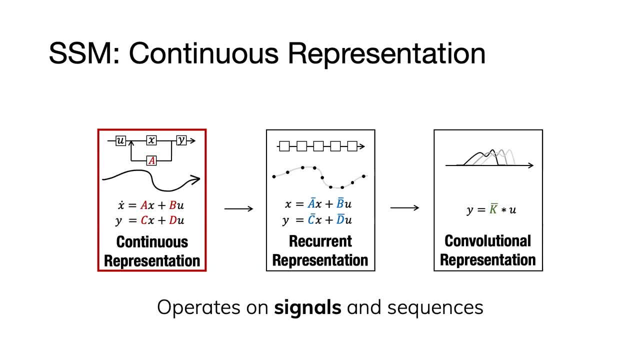 which is continuous, And so there's this fuzzy concept of inductive bias that this sort of like it just has better inductive bias for modeling certain types of data that are more continuous. Now the second view will be about recurrence, And so the motivation here is that 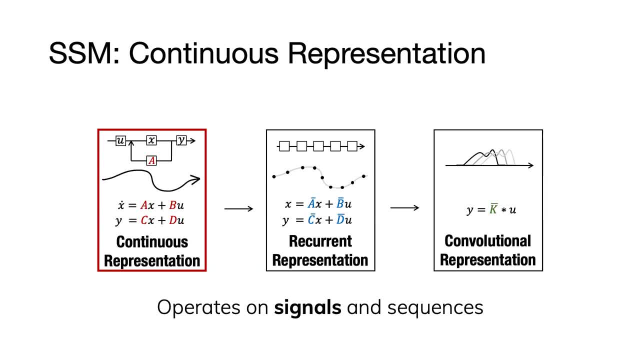 this is a nice representation that operates on functions, but in the real world, you always have data that comes in the form of sequences. right, You get that? time series that are sampled. So now, how do you make this model operate on actual sequences, which was our original goal? 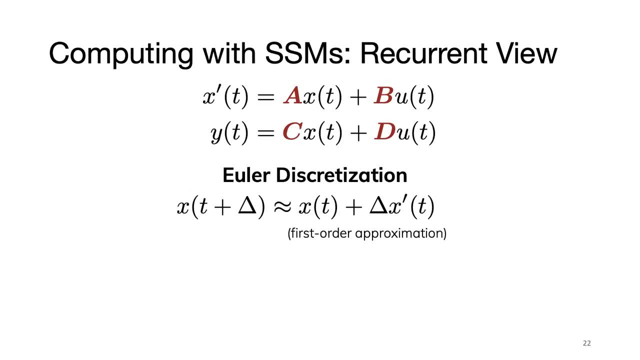 So what you need to do is discretize your differential equation to go from continuous time to discrete time. The way you do that is using these standard techniques called. there's a lot of discretization techniques, and you can really treat them as kind of these black box formulas. 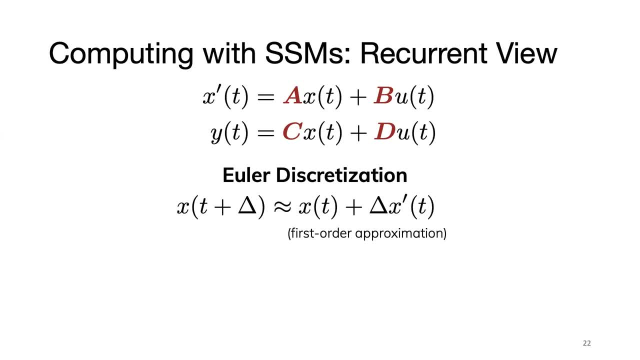 but just to really briefly illustrate the idea, you basically just approximate the differential equation- And there's a lot of standard techniques for numerical approximation of them- and then you can convert it into a discrete form. Here this is illustrating the most simple. 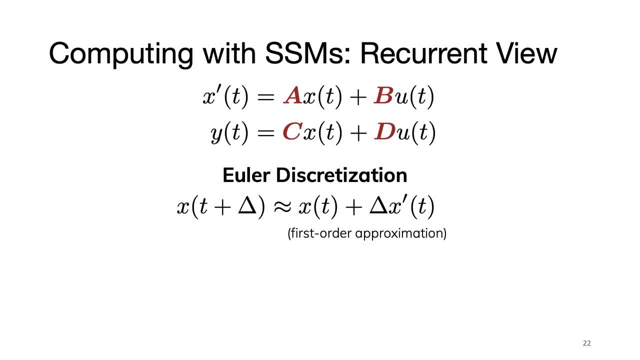 illustration. the example is called the Euler discretization. So basically you can think of simulating your differential equation by moving it forward, say like one second second at a time, And to get from your current step to your next step you just use this first. 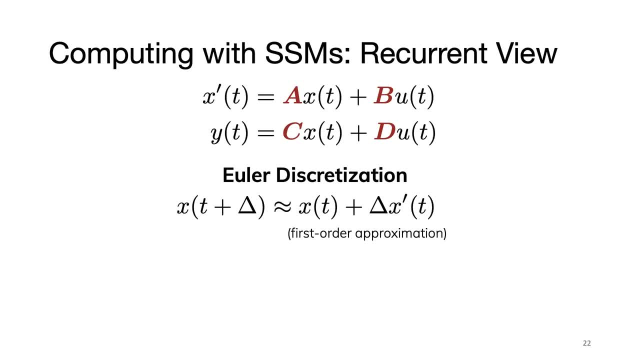 order approximation, to say that my next step is going to be incremented by the derivative of my function. So if you expand this out and plug it back in you, yeah. so you just take the derivative formula, differential equation, plug it back in and then you can get an exact formula. for what? 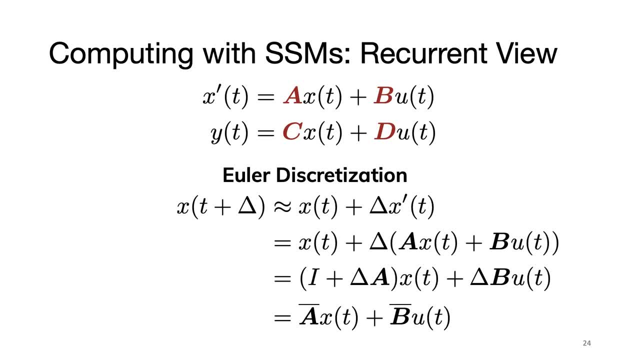 the next step of the sequence is going to be as a function of the current step. Yeah, this is recorded, so I'll actually not spend too much time here, because these equations are actually very simple if you just start them for a second. But the upshot is basically that you can. 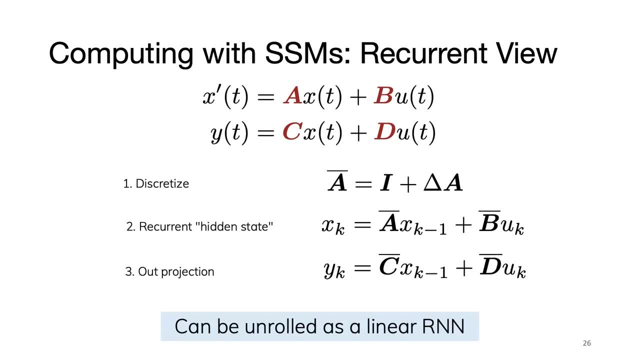 turn this continuous time model into a discrete time recurrent update. So the differential equation became. instead of becoming a differential equation, it got converted into a recurrence right here. So the second line here just says that, yeah, your next hidden state is going to be: 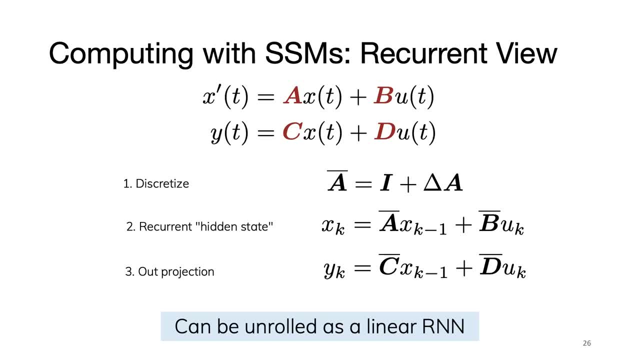 a linear combination of your previous hidden state and the incoming input, and then you project it back out, And these two equations are really basically just the essence of an RNN. So recurrent neural networks are basically defined by updating a previous hidden state recurrently and then projecting it back to the output. So you can basically view this as a very 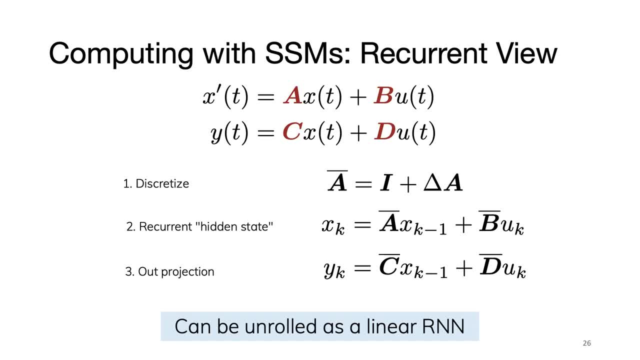 linear RNN, where the recurrent dynamics are given by this A matrix, and then there's a couple other parameters And yeah. so one thing to emphasize is that the underlying parameters of the model were A, B, C, D and actually this extra parameter, delta, which represents 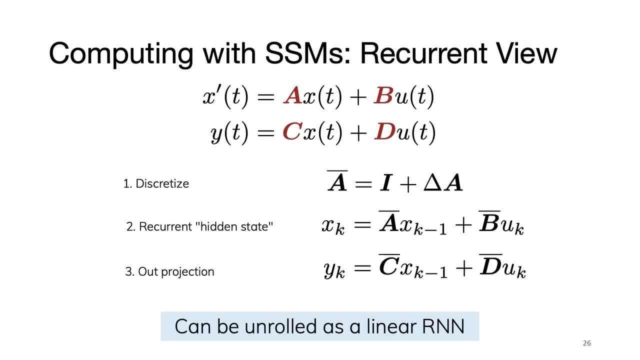 the step size. And then the first step in your computation graph will be to follow these fixed formulas to generate discrete matrices, A bar and B bar, And then those are the matrices that define the recurrence, which is what you will actually use to step your model and compute it. 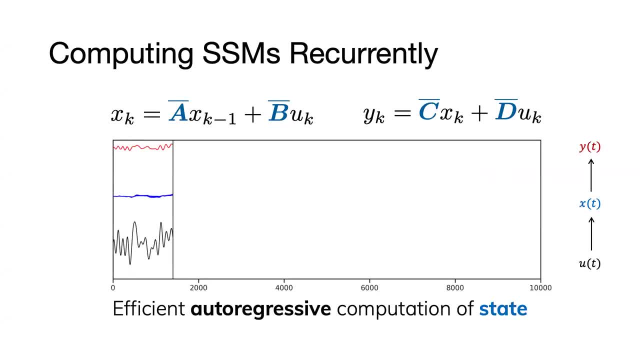 So I had some more intuition for discretization that I'll skip. So what's the point of recurrence? So, first of all, this gives us our first way to actually compute the model, When we get one input at a time, then you just update your state generate. 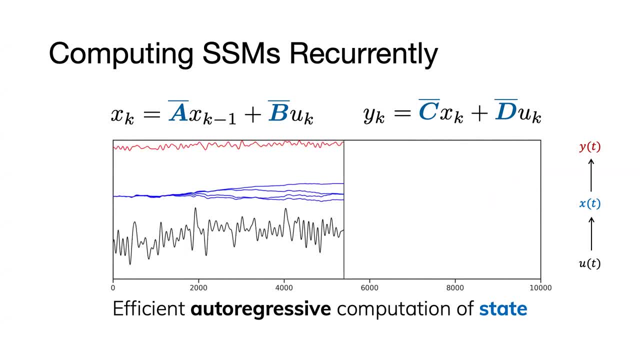 the next state, generate the next output. And, more importantly, RNNs have a lot of nice properties that other types of sequence models don't have, And that's because they're recurrent and they have this finite size state. So we all know about language modeling, for example, where models 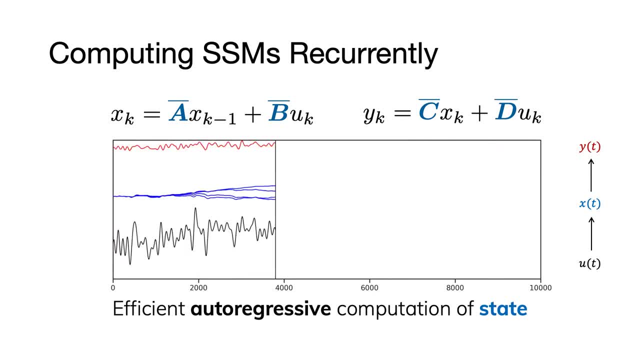 are trained auto-regressively, so they predict the next token. And when you want to generate something as a language model, you have to take your output and feed it back into your input and then pass it through the network again and feed it back in. So this auto-regressive 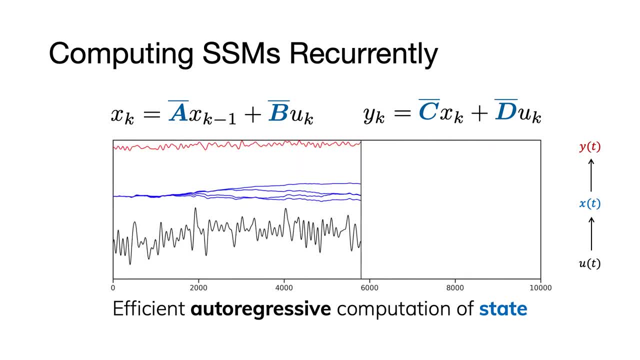 computation is recurrent and RNNs are actually much faster at doing that generation, just because you know it's a released output. so you have to do the same thing over and over and over, Moving back to the next slide, this step again, we went back to the parallel regression. 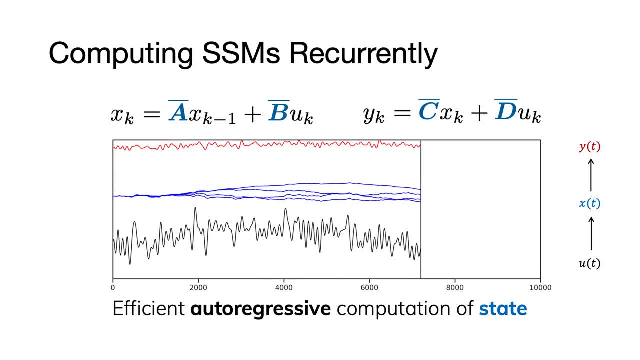 their hidden. their state size is constant and so every single time step takes a constant amount of time. um, actually, yeah, so this is an illustration of it. so let's say that we've seen like some amounts of the input and we're trying to we get one more input and we want to get, uh, generate one. 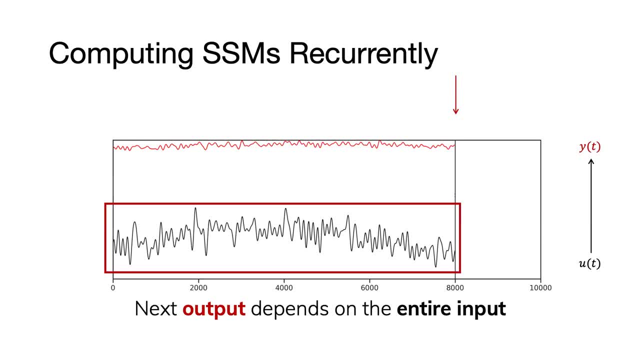 more output, um, this output is actually a function of the entire history of your input. it's not just like a, it's not just a function of the current time. step right, you're taking in the whole history, um, but despite that, and despite the input size increasing over time, every single output you. 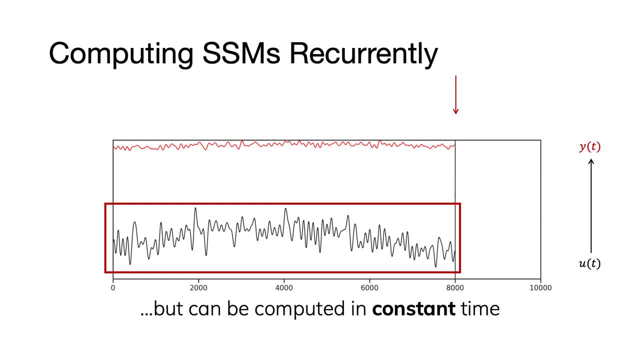 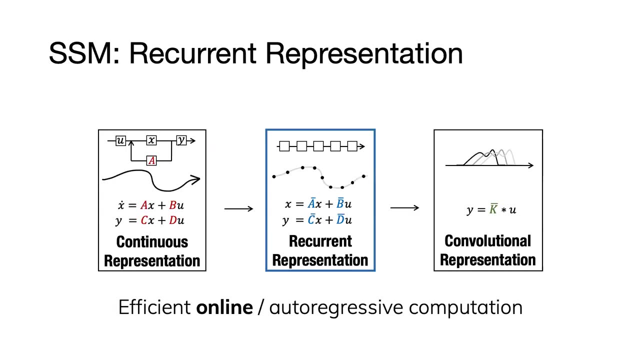 generate takes a constant amount of time. so that's a way to kind of illustrate why recurrence is powerful, um, and this is not true at all for things like transformers. so, um, a transformer model is going to slow down the more you, the longer your sequence gets. uh, so this is the second representation, which is basically um. first of all, how do you? first of all, 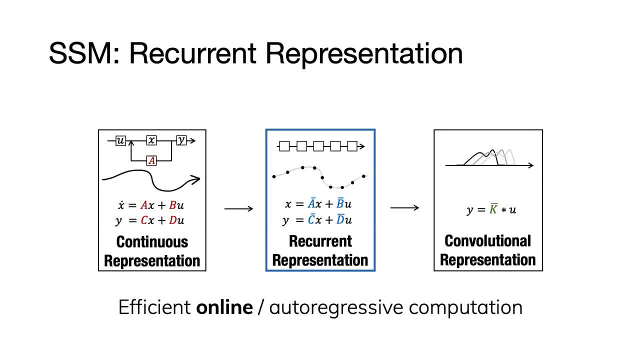 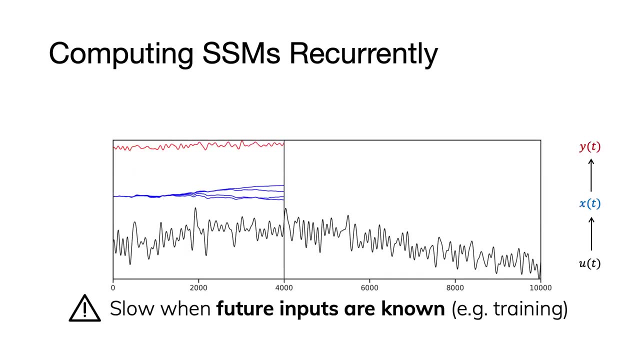 how do you take your model and your continuous model and make it discrete? so it's now. this is now an actual sequence and sequence map, which is what we wanted. um. and second of all, how do you compute it in a online or autoregressive fashion? um, now, the main downside of recurrence is that, if you actually know your entire input sequence in. 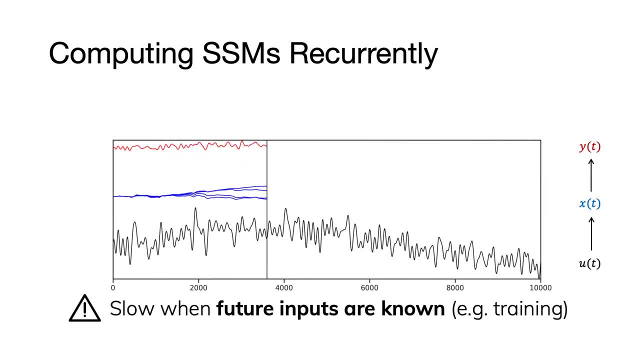 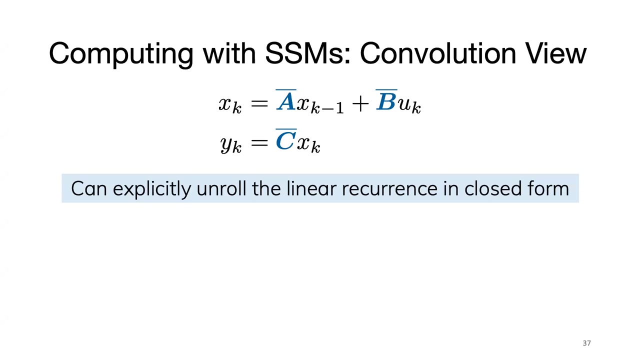 advance, then you. this is actually slow in practice, like on modern hardware: um, because it's completely sequential and you have to unroll this one at a time. um and modern accelerator with列's again and again. I dropped the D term because it's very easy to compete with the D term, so we can ignore it. 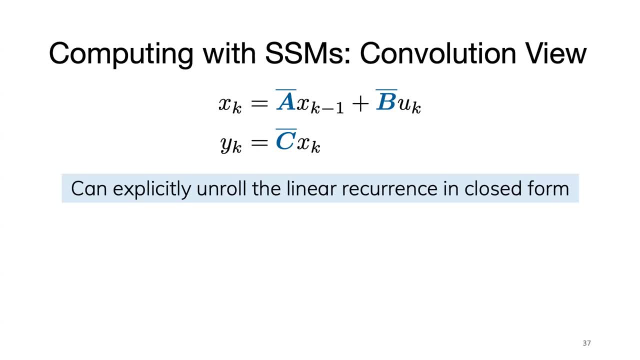 But yeah, here again is just the recurrent formulation And you can basically unroll this in closed form. So your first state x is going to be this: b, bar, times the first input, u, u0.. Then you multiply the whole thing by a bar. 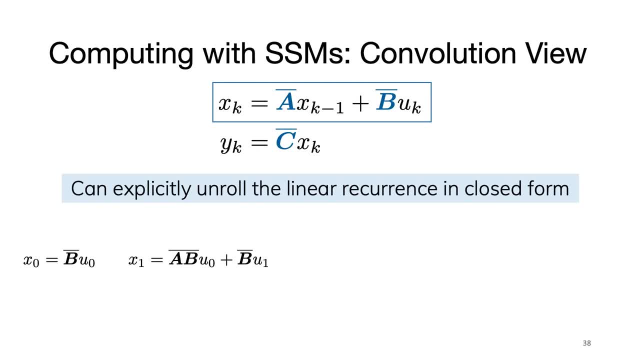 and add the next input by iterating that box equation And then to compute x2, you multiply the whole thing by a bar again, add the next input. So basically you can just continue iterating this. And the second equation is just a linear projection of this. 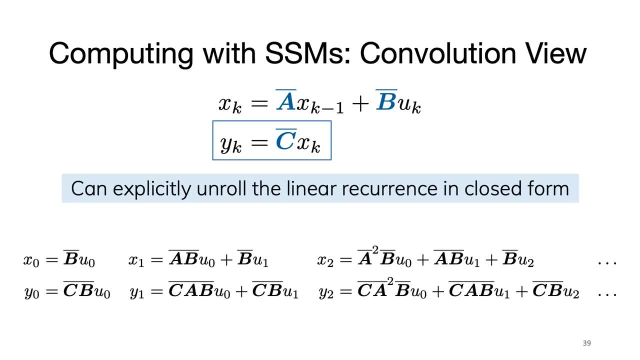 So the formulas are again very simple And the takeaway is that your outputs. so again, this is a map from the sequence u to the sequence y, And the point is every element of the output sequence. you have a closed formula for it in terms of the input. 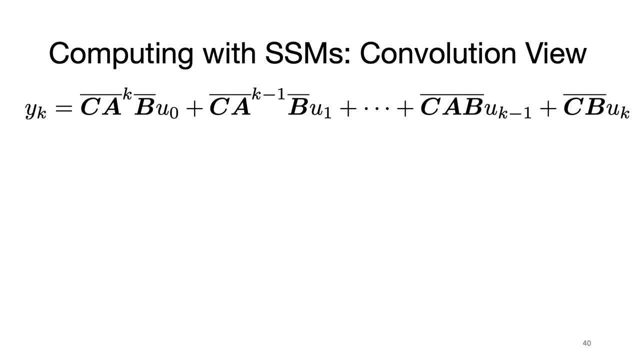 This is the general form. So, without needing to unroll the recurrence on the machine, you can basically unroll it analytically in equations And every yeah. so you know what the output is as a function of the input exactly. And if you look at this, you'll notice. 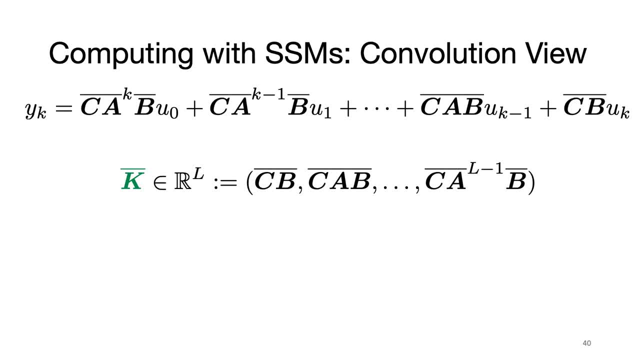 that it's actually a convolution. So this is the full equation. So the way to think about this is that I had my SSM parameters a, b, c. I discretized them to a bar, b bar And c bar is actually just c. 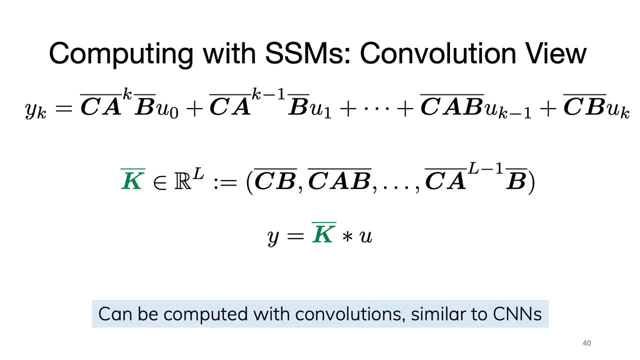 And then you can use that to define by, just by computing this formula right there. This defines a vector called k bar, which is the same length as the sequence, And k bar is basically what we call the SSM convolution. So you can use that to define a vector called k bar, which is the same length as the sequence, And k bar is basically what we call the SSM convolution. 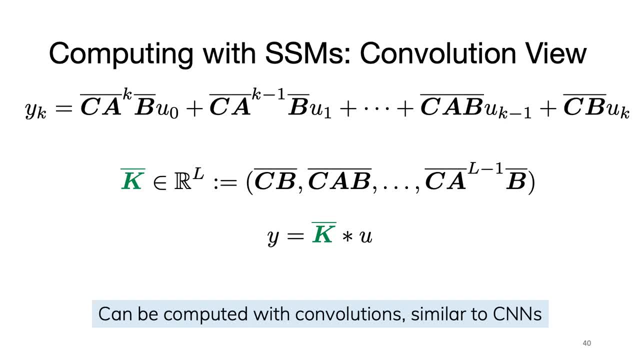 So this is the very simple convolution kernel, because the output y. so this is a map, the SSM is a map from u to y And the output y is just a single convolution of the input with this particular convolution kernel. So this is actually, I think, one of the easier ways to think about the model, or like the 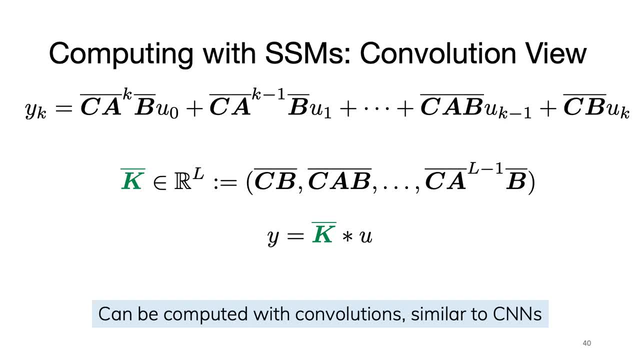 the cleanest way to relate it to classic learning architectures, because basically you can, just you can, think of this deep SSM as basically just the same as a CNN, or it's a. it's a variant of a CNN, where the convolution kernels are just parametrized. 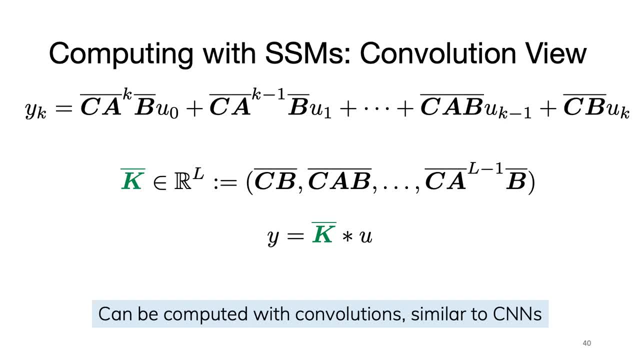 differently. so instead of defining a convolution kernel using a finite window convolution where every element has a parameter, these are sometimes called implicit convolution kernels or implicit CNNs, where it's again just a CNN, but the convolution kernel is defined implicitly through this formula k-bar. that is a function of the actual underlying parameters a, b, c. 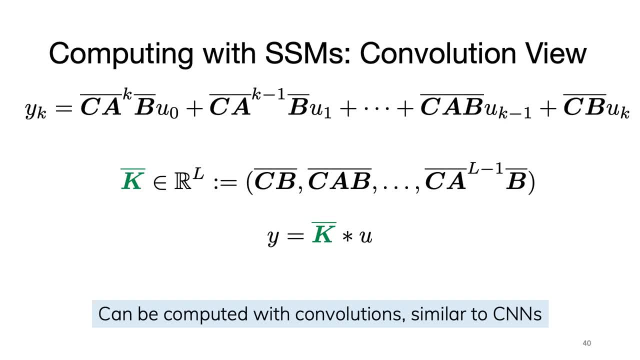 and one motivation for that is that this convolution kernel is actually infinitely long. so what? and this kind of relates to one of the some of the properties of SSMs that we'll see, which is one thing that the S4 model was originally known for, was being able to handle really long. 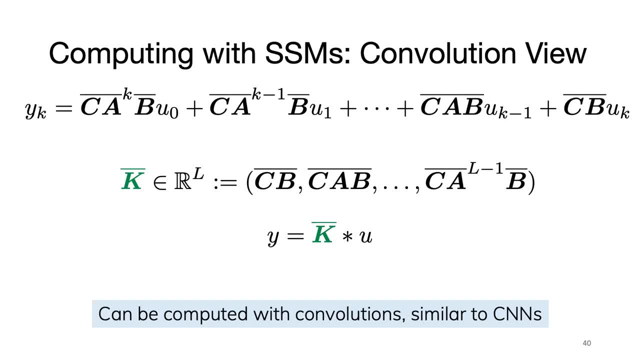 sequences and one way to think about that is: well, all of the, all of the views shed some insight into that. so, as an RNN, RNNs have an infinite context because you have a state that just keeps getting updated through time. and as a CNN, you can also see it because the convolution kernel is infinitely long. so 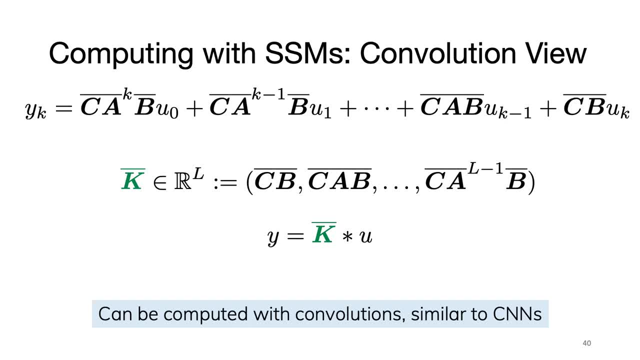 the model is kind of attending to everything in the past, but now, if you want to parametrize an infinitely long convolution, that's clearly impossible and thus it's a. it's a formula that's based on some compressed parameters, so that motivates. that's another way to think about this. 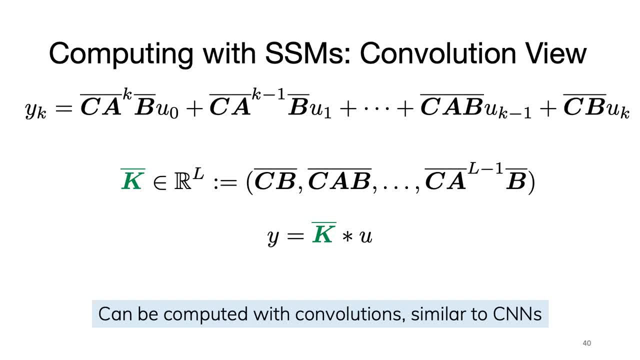 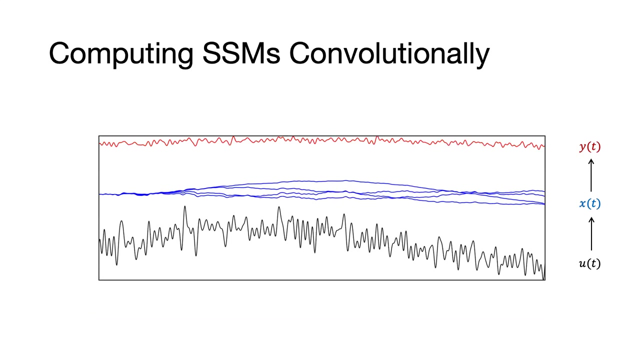 implicit convolution. um, yeah, any questions about this, like the RNN we've seen in you. okay, so that's. oh yeah, here's another illustration of it. so, um, the SSM was a map from the input u to a state x to an output y, and um, the way that. 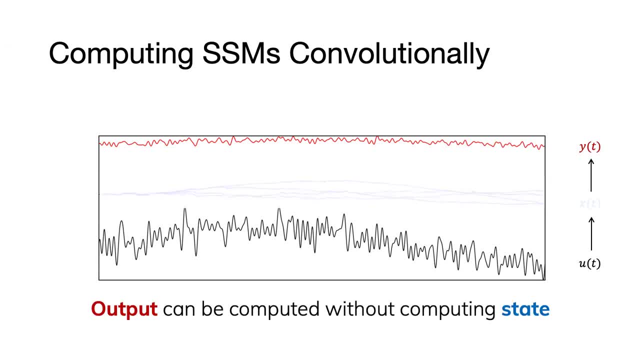 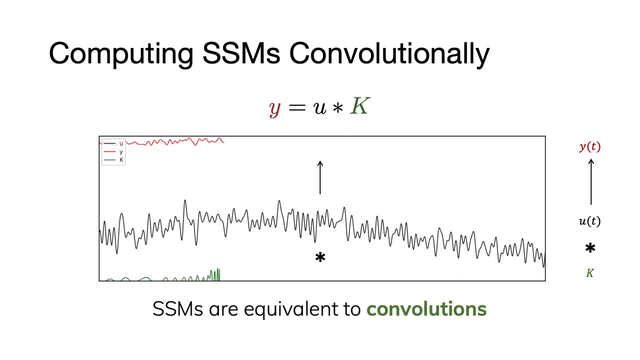 it kind of works as a convolution is that instead of computing these three things one at a time, you actually can completely skip computing the state and write the entire output as a convolution of the input, with this particular convolution kernel, which is illustrated in green here. 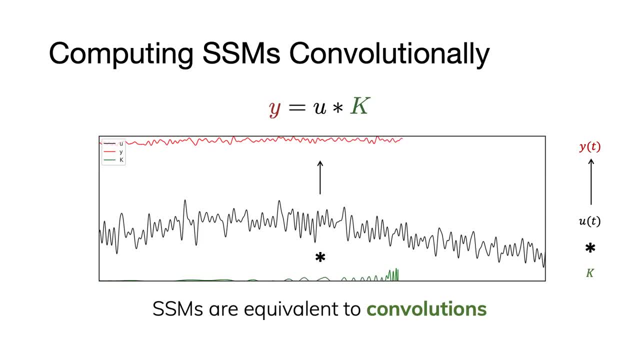 And this is just a standard convolution. You take an infinitely long convolution kernel, the green one, and then you're sliding it along the sequence and taking a dot product to generate every output. So this is kind of like another way to do the same thing. 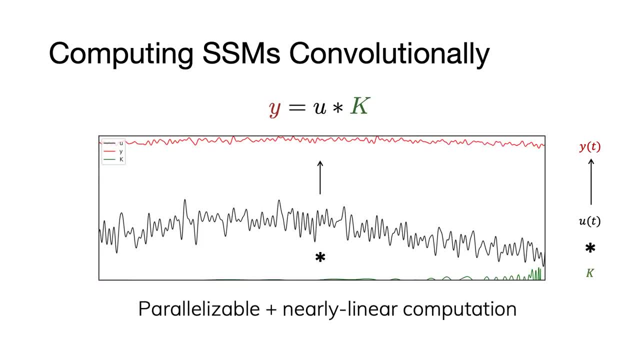 But the benefit of this is that convolutions are a very well studied object and you can compute this whole map If you have the entire input and the entire kernel, you can compute this whole map very fast using standard techniques like the fast Fourier transform, And so this overcomes. 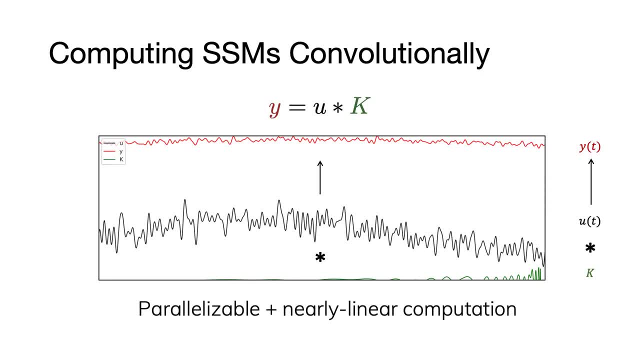 the original issue we had with recurrence of sequentiality. So this whole thing can be computed in parallel Over the entire sequence length and quite fast on like GPUs. Yeah, great question. So the kernel is actually implicitly infinitely long, as I mentioned. 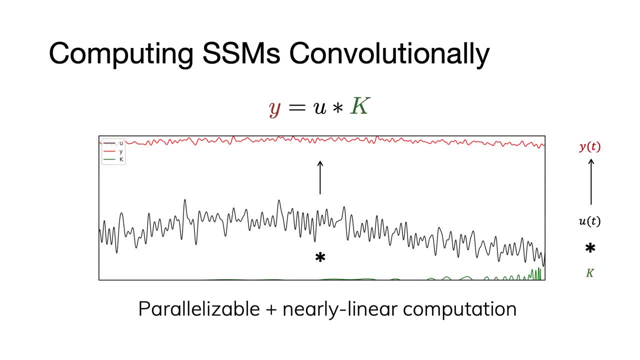 But if you have a finite sequence of length L, when you convolve it by an infinitely long kernel, it's the same as truncating the kernel to the same length as the sequence, because the rest of the kernel will never be dot product with anything. 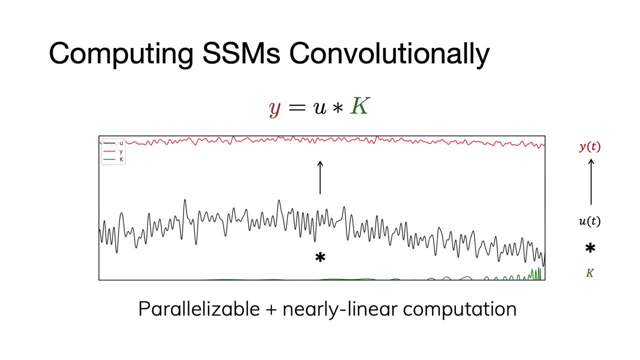 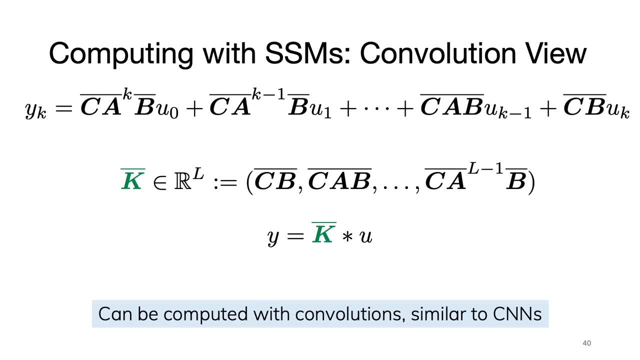 right. So basically, in practice, what happens is that you take the input length of your sequence, which is capital L here, and then we're going to define the convolution kernel truncated to that length and compute just that kernel using some special techniques. 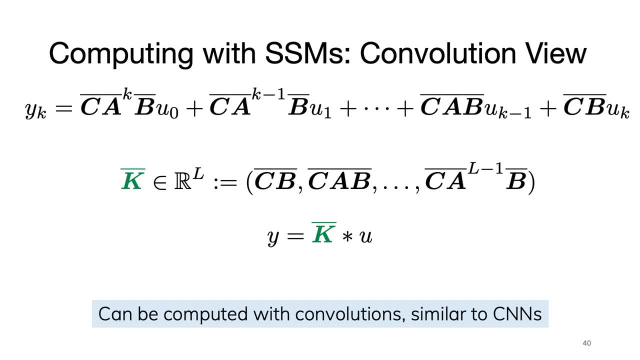 Yeah, Yeah. so for this basic model, the model I'm showing here, it's actually a particular flavor of SSM called time invariant SSMs, which have this dual view of recurrence convolutions, And the point to emphasize is that they are computing the exact same model. So the trade-offs between 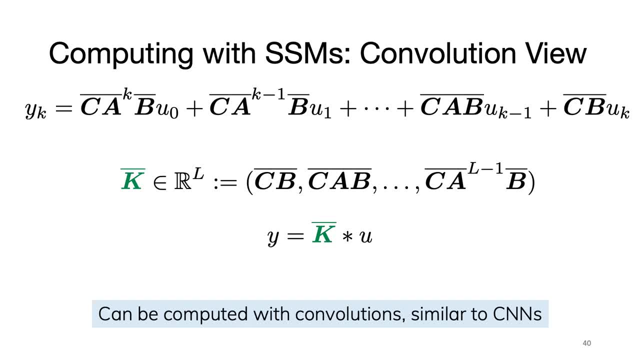 these are all about the computational trade-offs, Yeah, And the computational trade-offs basically are for this original model. basically the trade-offs were that during training time you generally want to use the convolution view because you see, normally during training 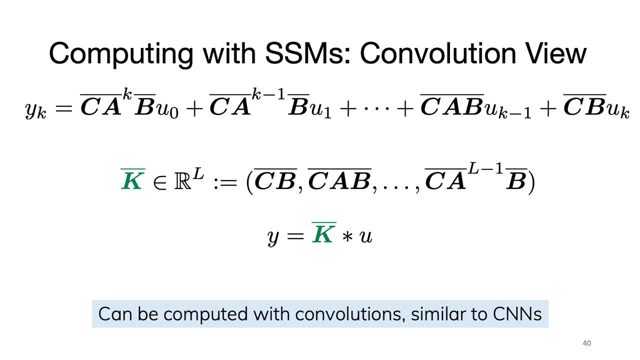 you see an entire batch of your entire sequence and you want to do this computation parallel, So you can compute the kernel and then use the convolution to compute the whole map. Yeah, So if you look at this particular model here in the прекрас, for example in language modeling, 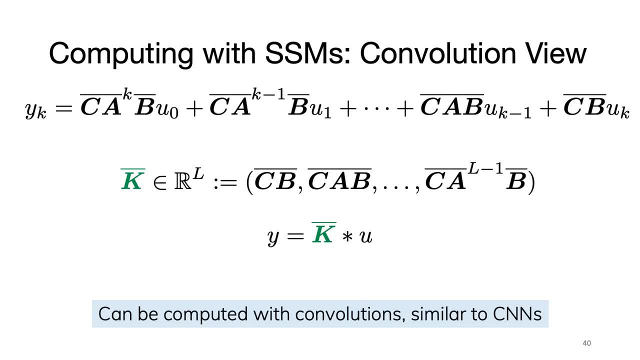 even though the objective function is auto-aggressive, during training you actually see every single element of the sequence at the same time because you use what some people call a reversed teaching forcing. So you do always want to use the convolution view in general. The recurrent view generally you only want to use in settings where you need to be. 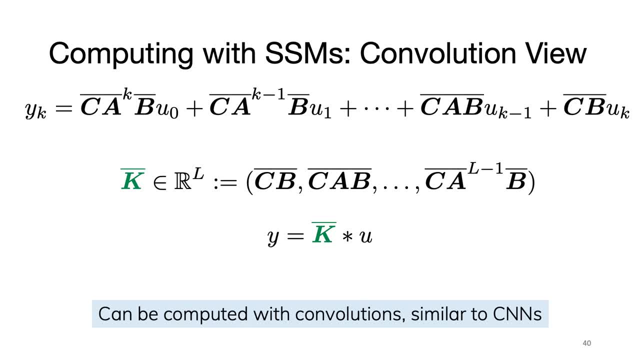 auto-aggressive or online. So some settings include: Okay, Okay, Okay. modeling is an example where, during inference time, you'll want to use the RNN. Other settings, like reinforcement learning, might be similar, where your actors might want to be they kind of. 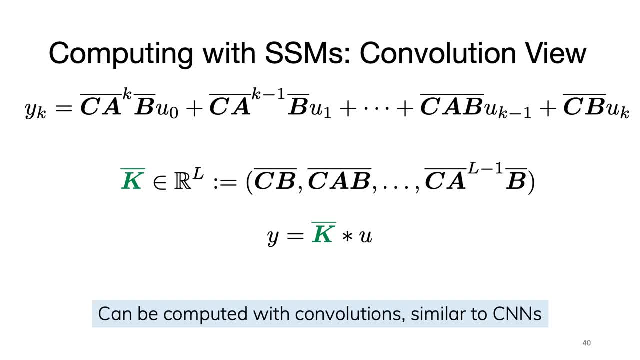 like when you do an action and then you get a new observation and then you- only then- can you do the next action. So anything where you're not seeing the sequence ahead of time you'll need to use the recurrence, But otherwise the computation is generally faster. Now there is a caveat. 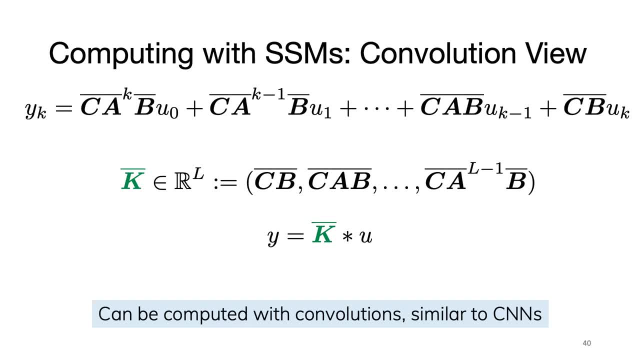 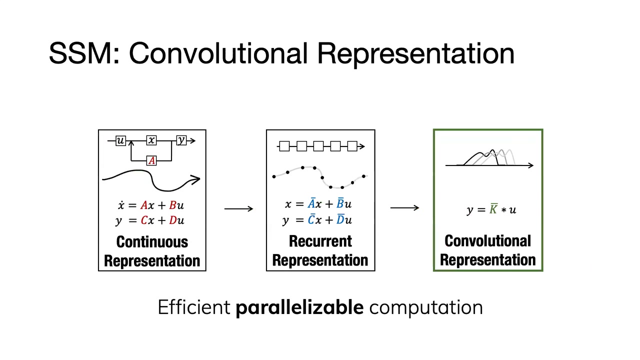 which is that there's active research in figuring out how to make the recurrent view faster, because it's actually more flexible in some ways. But that's ongoing research. Yeah, did that answer your question? Okay, Okay, Yeah, so that was about the convolutional view, which is about parallelizable. 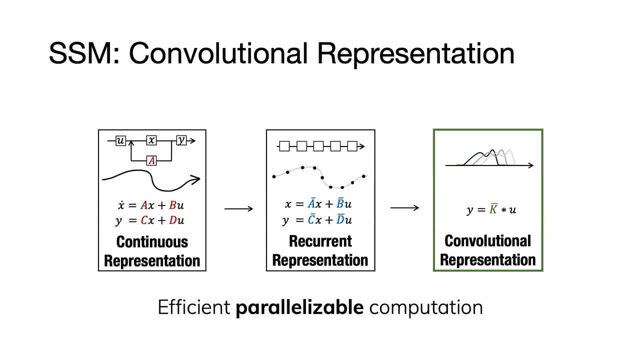 convolutional view. So that was about the convolutional view which is about parallelizable convolutional view. So that was about the convolutional view which is about parallelizable computation. Yes, on my question. so what is your interpretation of the latent state for these models? 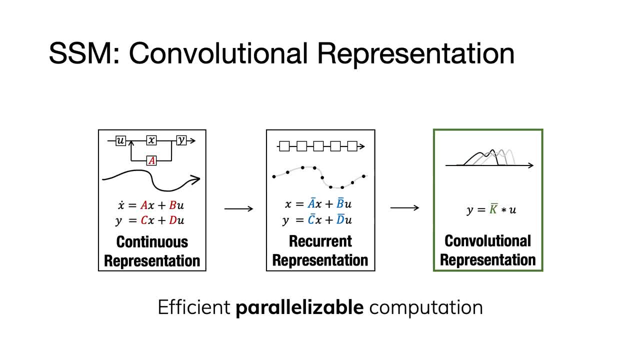 Good question. So that's actually kind of going to be the subject of the next part, which is the original S4 model: how to define these in a way to have a very particular latent state In general. so, more generally though, you can define SSMs without the extra stuff, like just 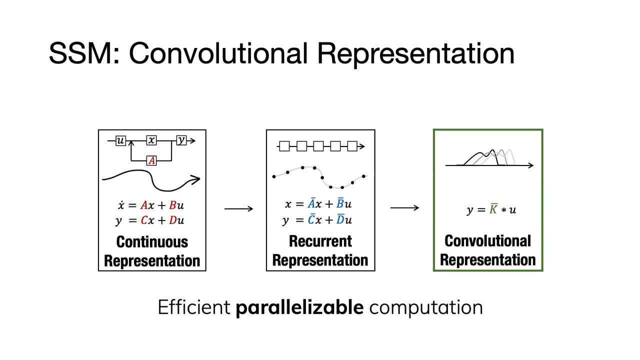 basic SSMs. I don't know what sort of interpretation you can look for. There's lots of things, But as an RNN, usually there isn't necessarily a clean interpretation of the state In this case, because it's a linear RNN and you can impose structure on it. you can come up with special 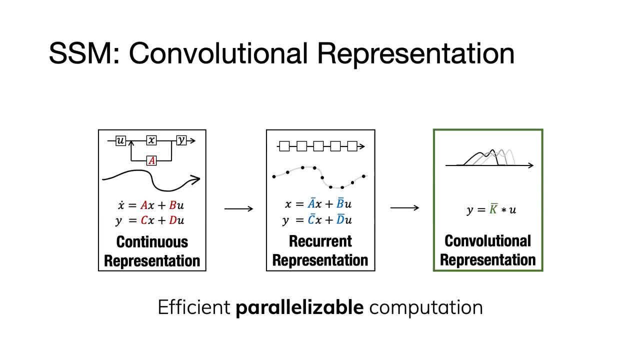 things that have nicer interpretations. For example, when you have a diagonal SSM, you can have a linear RNN and you can impose structure on it, And you can come up with special things that have nicer interpretations. For example, when you have a diagonal SSM, you can have a linear RNN. 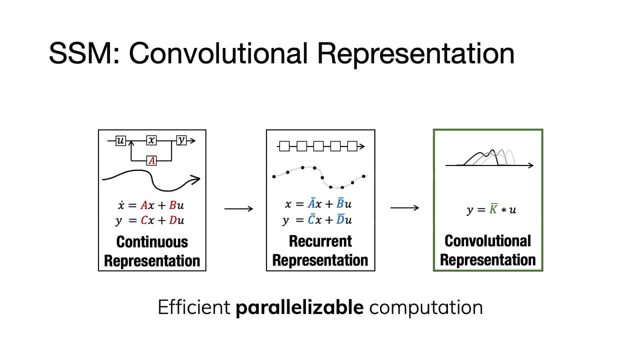 which we'll see a little bit later. you can view your latent state as kind of defining dynamics that smooth out your history at varying rates. Another interesting thing is that you can actually view a local CNN as an SSM where the A matrix is like a shift matrix. 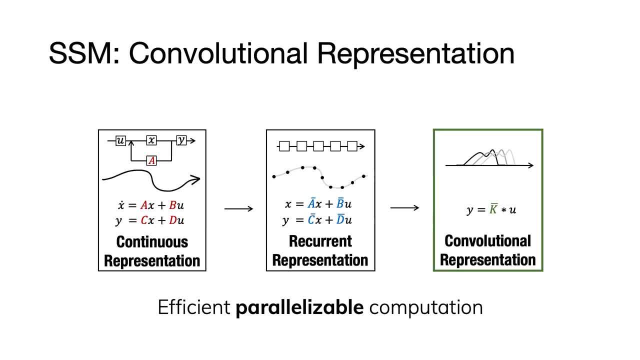 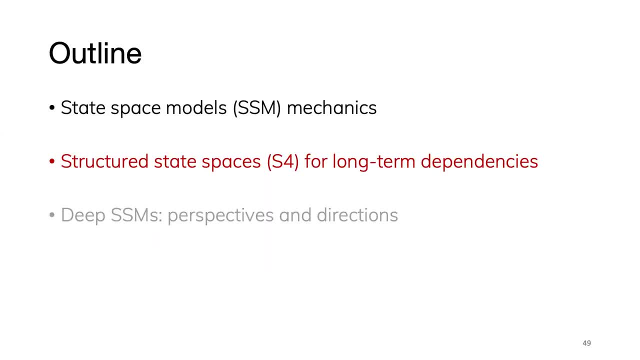 and you view the state as kind of just a buffer of your history. So basically, every single different SSM will have a different interpretation. The next part we'll see is going to have a. the original S4 model has one very particular interpretation. 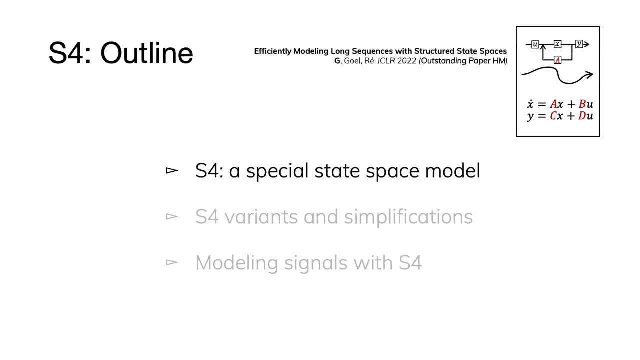 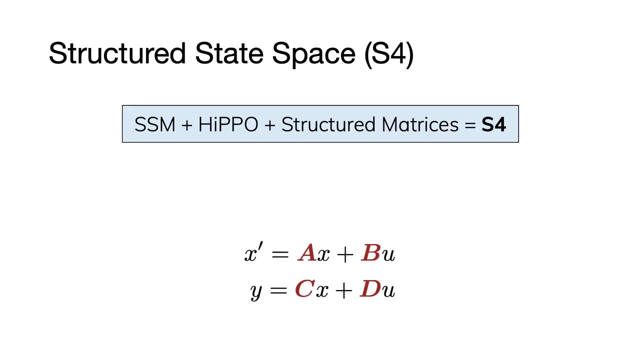 So yeah, so let's talk about S4 now. So you can basically view this as a particular case of these, of a state-based model, And to define it, the definition is actually very simple. We're gonna take this basic SSM that we saw. 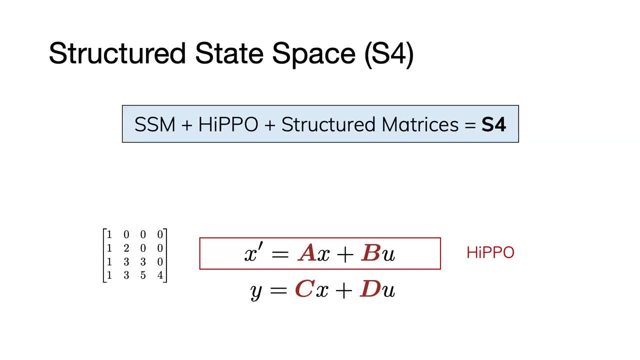 and now we're gonna use special formulas for the A and B matrices, which are called HIPPO matrices, And that's pretty much the whole definition. It's just an SSM with special matrices for this. but also to compute the model you're gonna need to use some very bespoke algorithms. 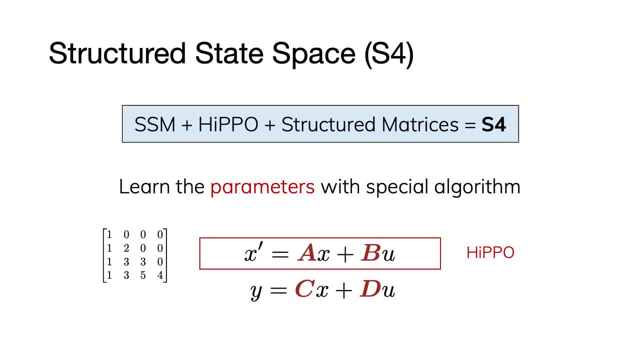 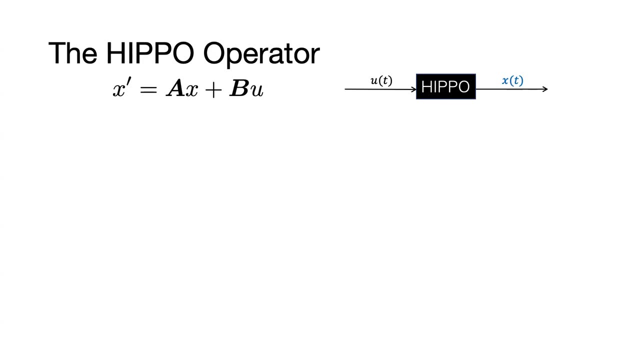 to be able to compute this efficiently. So we'll kind of now we'll go through both of these. So first, why, what are these matrices and what did they do? Okay, So HIPPO basically is a particular definition of the first SSM equation. 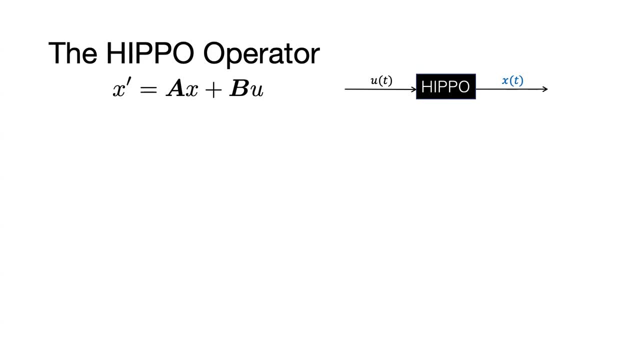 So again, it's giving you like. it basically specifies fixed formulas for A and B And, and just to recap how to think about it, HIPPO is a map from the input u to a state x, And it was motivated by the recurrent view. 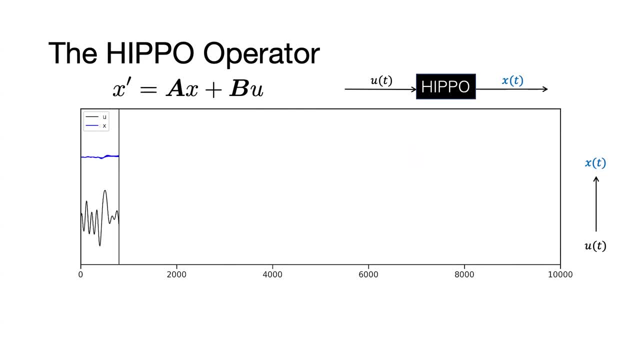 So the motivation is: it's essentially, if you are taking this equation and you're getting new inputs and you're updating your state, can you come up with a state that has a very meaningful interpretation? And, in particular, the motivation of this was: can you design a state that is actually capturing? 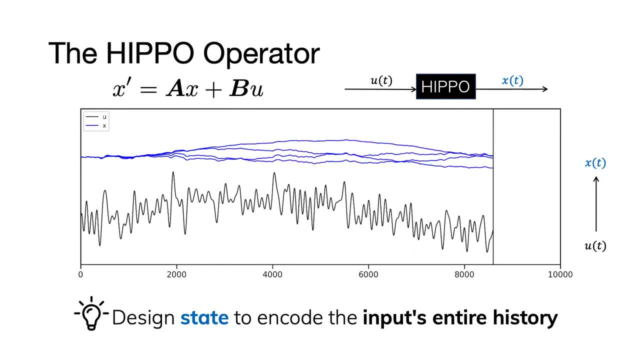 the input history in a way that allows for long-range memory. So the original motivation was to address long-range dependencies with RNNs, where RNNs were famously known to suffer from addressing long-range dependencies, And so HIPPO was kind of. 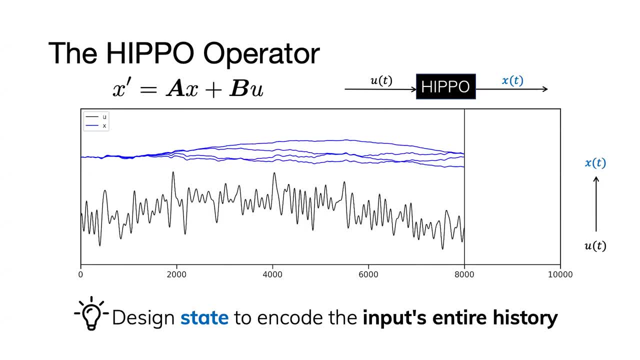 from an RNN perspective. how can we do this in a principled way And the way the the motivation was just to design a state that can capture the input history, which should should allow you to have long-range dependencies. And more specifically, let's look at the setup. 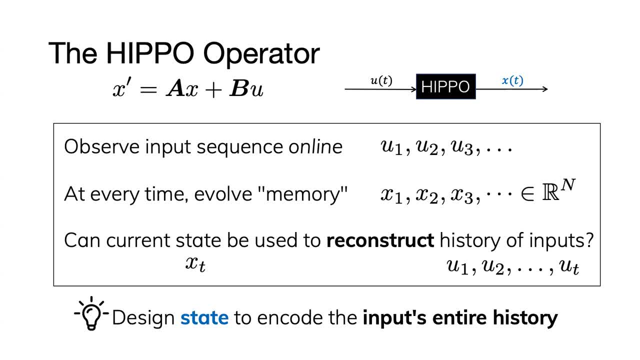 So we have an input u that we're observing one time, step at a time. So each u1, u2, u3, these are just scalar numbers And every time we see an input we're updating our state x, which was this fixed length vector of length n. 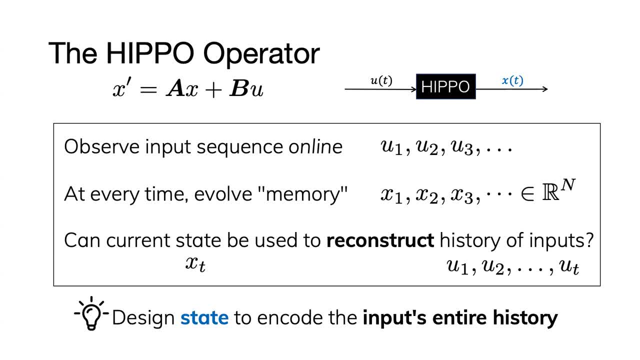 And we asked the question at every given time. step t: we have a state x of t, which is a vector, And can this state be used to reconstruct the entire history of inputs we've seen so far? So I think this is a very natural question. 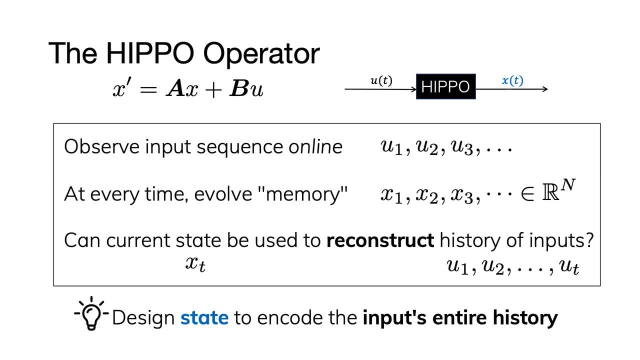 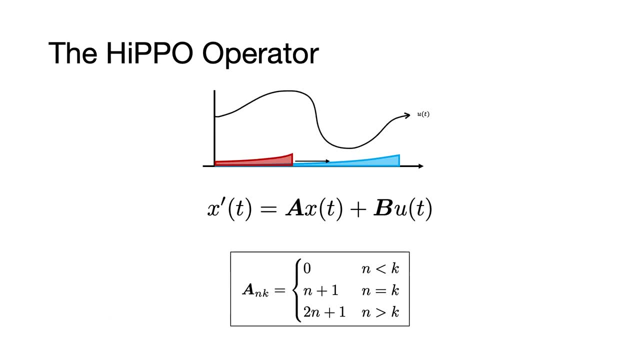 And we call this online function reconstruction, because you're getting an input function and you're trying to reconstruct it online. So the answer is, of course, yes, you can do this, And that's where the formulas came from. So the answer to like: how do you do the reconstruction? 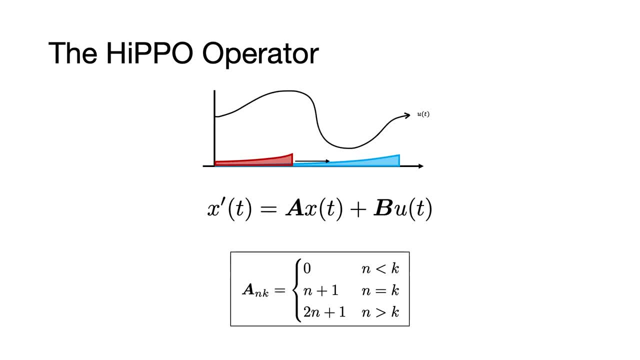 So, basically, this equation was the thing that answered that question, And we're gonna work in continuous time, So the question now is: given an input function, u, that you're observing online continuously, what are some dynamics of the state that will allow the state to evolve in a way? 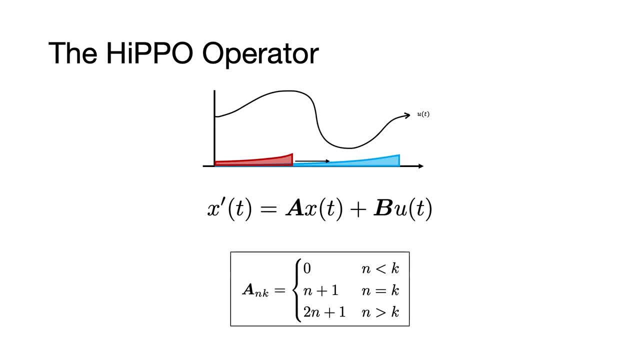 that's continually maintaining some memory of input. So the way that it evolves is exactly this equation- the first order linear differential equation, with some particular formulas for the matrices. So I'll illustrate this in just one second. Well, just for terminology, this differential equation is what we call the Hippo operator. 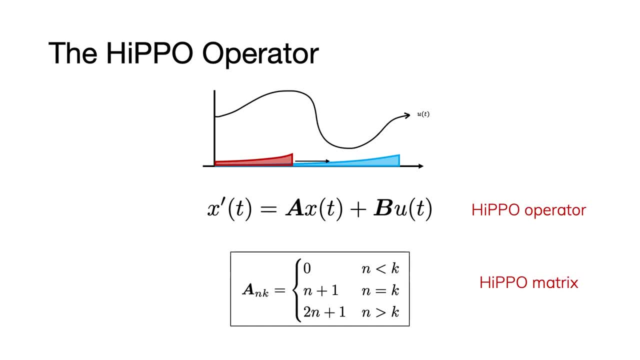 And it's an operator, because you're thinking of this as a function to function map, where you take this input u of t and Hippo is gonna map it to this higher dimensional state x of t. that is an online compression of the history And the matrices here in B are called Hippo matrices. 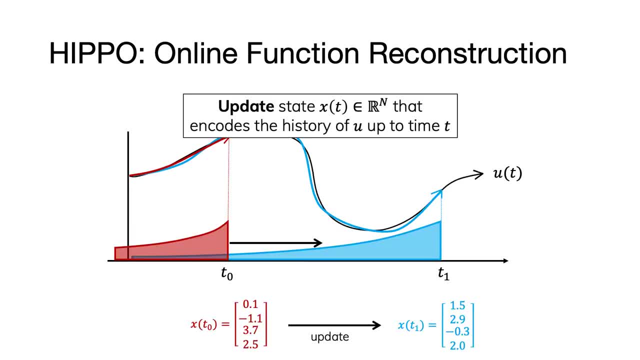 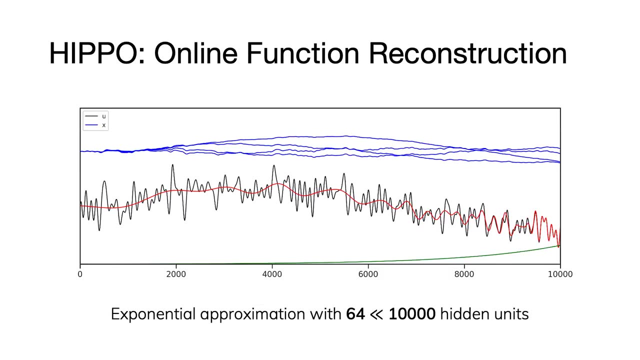 and A is the more important one, Okay. so, oh, actually I had sorry- Yeah, I had some more slides that I skipped- that kind of illustrate the process in more detail, but let me skip this, Okay, so let me just illustrate. 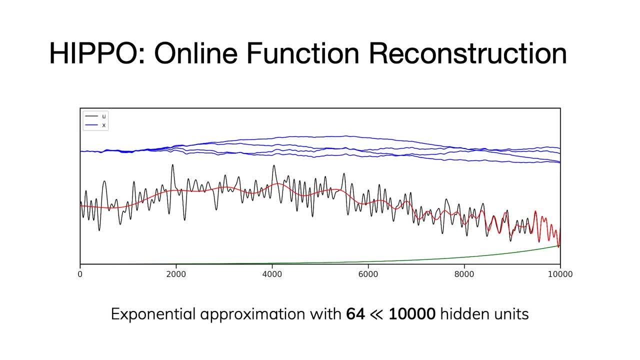 what does this actually look like? Okay, So here we had this. I have the same function, u, that I've been using, the black line is u, And now we pass it through Hippo, which gives me this state: x in blue. 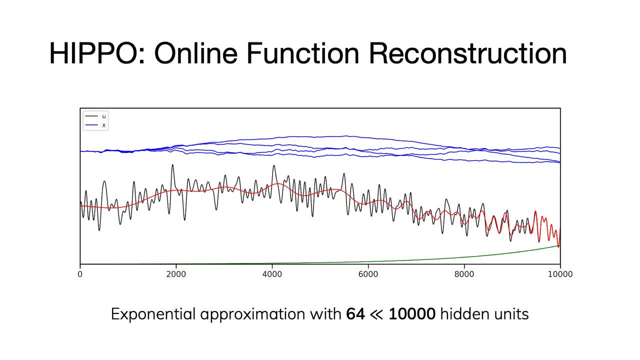 which you can think of as actually we're generating this, we're currently online And I'd illustrate the function reconstruction aspect. If you look at the last time step, I consumed this input sequence of length: 10,000.. And in this particular illustration, I've used a. 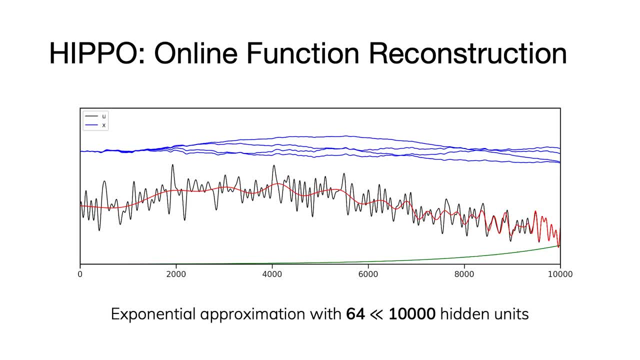 a hidden state of size 64., So that capital N was 64.. I've only illustrated four things just for make it clean, But what I used to generate this had a vector of length 64.. At the end of the whole thing. 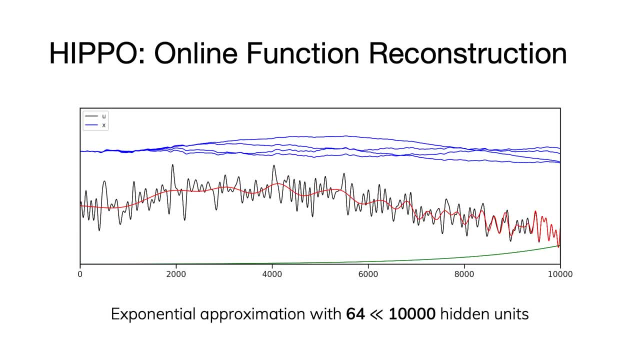 I've consumed my entire input sequence updated my state and I now have a vector of length 64 in memory And I can use by a linear projection of that 64 numbers. I can use a formula to project it back out to 10,000 numbers. 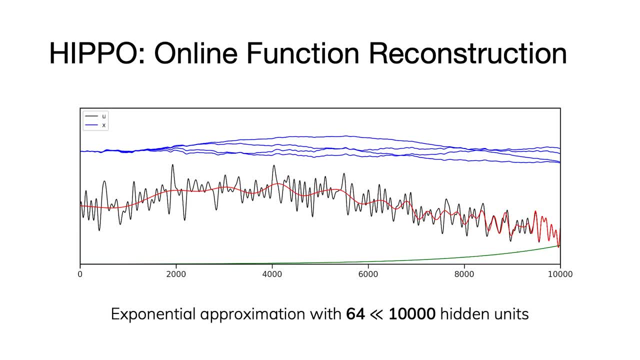 And that's the red one. So you can see that obviously, with the finite size state, we can't remember the entire history of the input, And so the question is like how, what sort of approximation can you make to it? And that particular formula I will show in: 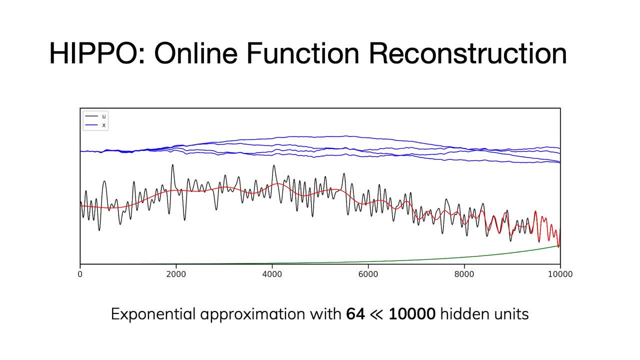 is giving you an exponential approximation to the input. So you can see the red line is. it's very accurate for the recent past and it decays out to the far past. More formally, the framework involved was prior or hyperparameter, that we call it a measure. 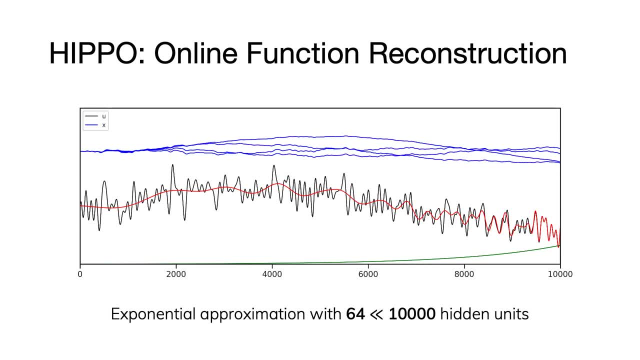 which is illustrated by the green line, which says: if I'm giving you a reconstruction and I want it to be a good approximation, how do I measure the quality of that approximation? We needed to find a root function that says: how much do you care about various parts of the input? 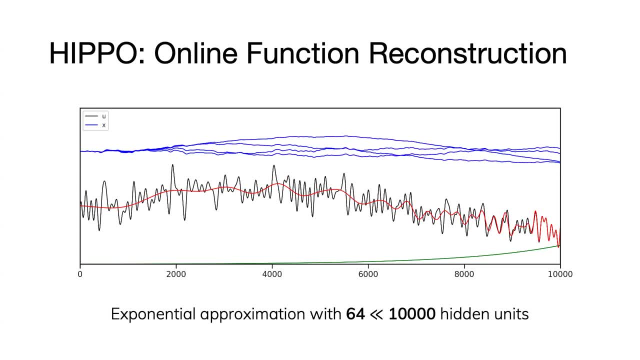 So here this green line, this green one is the exponential measure which just says that I care about approximating this part more than that part, So that's why the reconstruction looks like that. And now the more interesting part is that this was all motivated by doing this in an online way. 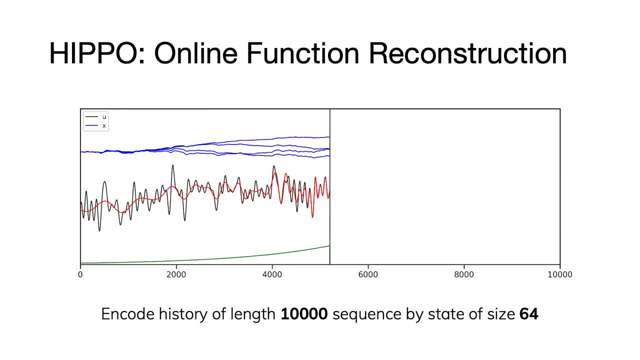 And that means that if I am observing the input, one at a time, I'm constantly updating my state, which are the blue lines, And at every single point in time that state can be used to give me that reconstruction And you can see how the reconstructions evolve through time. 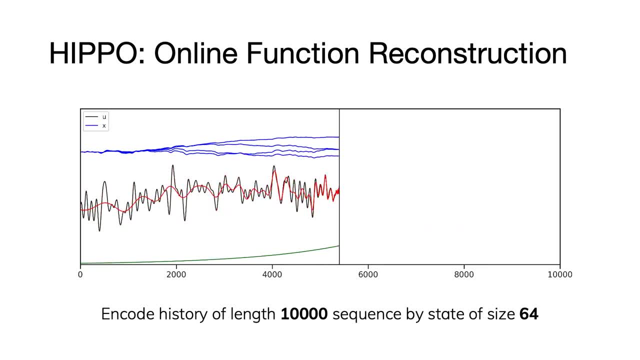 So at the beginning it's very accurate And then, as you move on, you're going to be remembering the current, recent history better and kind of losing, forgetting and losing a little bit about the past, But you're still maintaining some information. 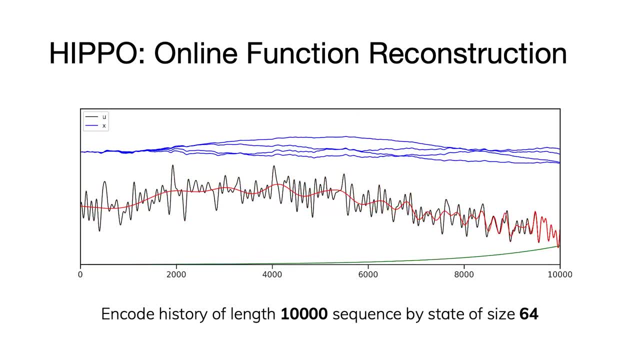 about the far past. Any questions about this? And yeah, so this kind of answers the question in chat about what does the state mean. So again here with S4, which is going to be based on hypo, the state is a compression of the entire pass of the input. 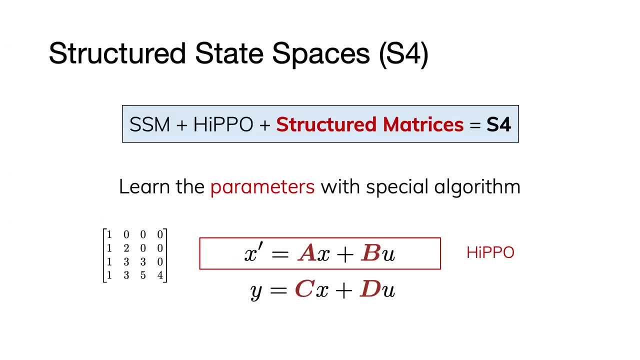 And this was motivated to give you a long range dependency, Because once you project it back out, you're hopefully able to leverage this information from the past. Okay, so that's the definition of S4. It's just plugging in these formulas into the SSM. 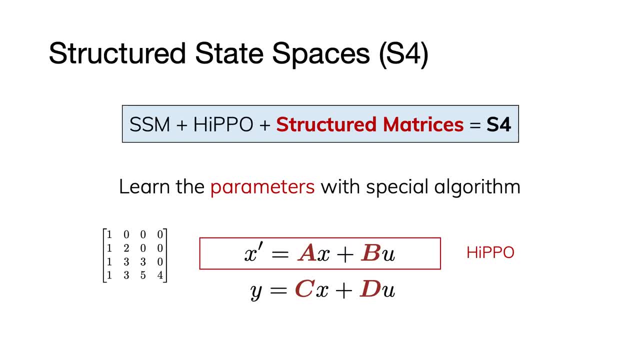 Now the issue is that actually computing this SSM is actually quite non-trivial. I skipped over some details earlier, So now why is it hard? Let's look at this SSM again And again. you can see here that the beautiful red line 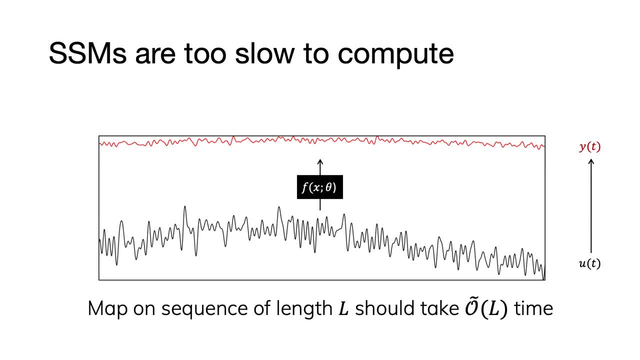 is a lot more of a transformation point, And so, again, it's a parameterized app from a 1D sequence to a 1D sequence. Here I'm using a function view, But yeah, just assume this has been discretized to a length L. 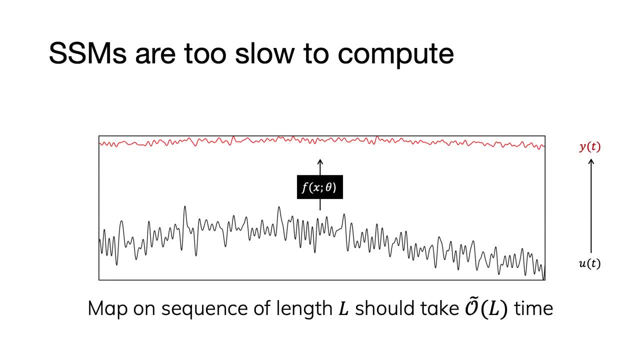 This map is consuming a input with L numbers, which is the input sequence, And it's outputting L numbers, And so ideally this should take L time or not too much more. So if you look at things like normal RNNs, they scale linearly with L and so on. 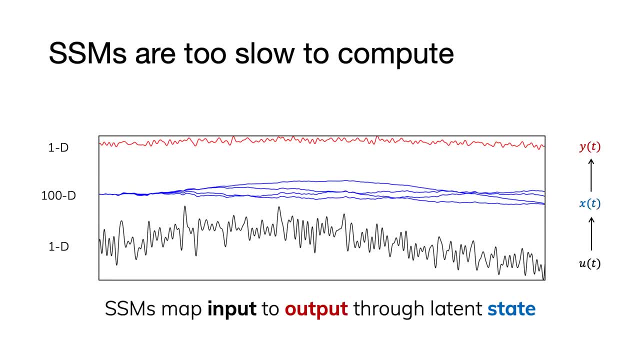 Now, if we look at the SSM, remember that it mapped the input through the state X, which is higher dimensional. In the previous HIPAA illustration I had: N equals 64.. In general, you're going to want something maybe on the order of 100.. 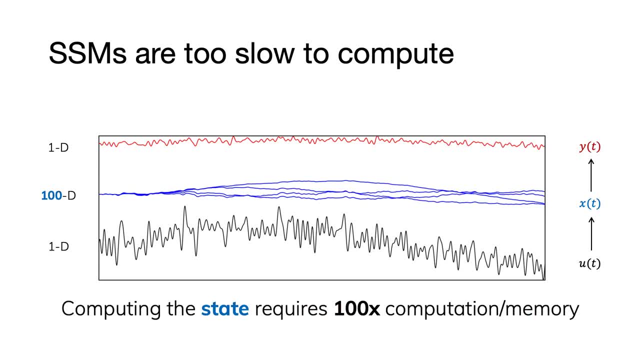 And if you think about it, that means that when you do this computation, just materializing That latent state is going to be 100 times L- numbers that you have to store in your memory, And computation-wise it's also going to be at least 100 times L. 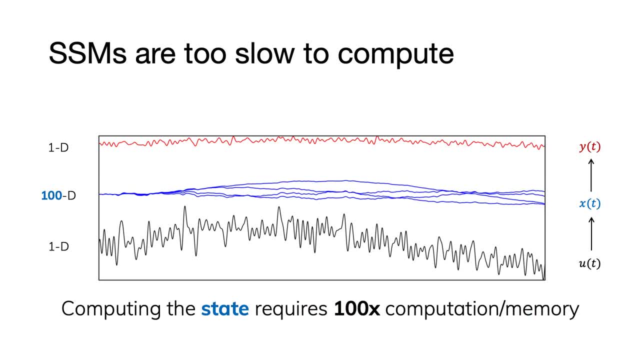 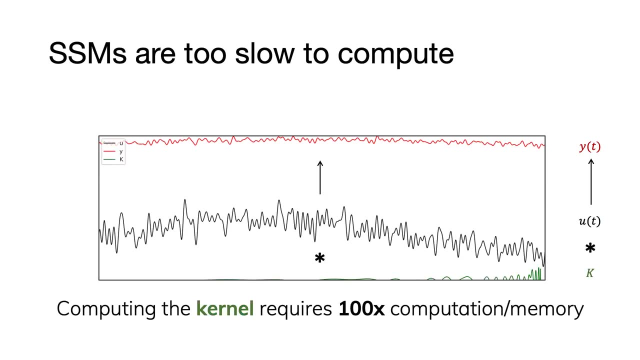 So, more generally, basically, you're going to need O of L, space and time just to materialize the state, which is a lot more than the bound here. We want to just L, And now I mentioned there's a separate view. 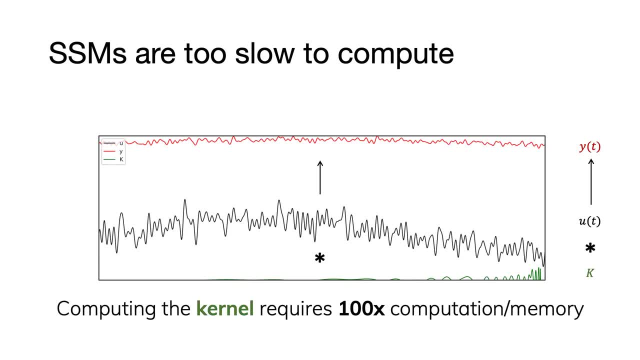 There's the convolutional view, which allows you to bypass the state, but the hardness of the problem still remains. In this case, the convolution itself is fast, but computing the convolution kernel is going to be very expensive, So there's no free win here. 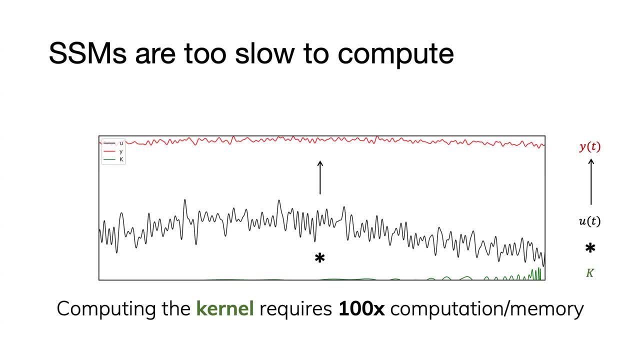 One way you can do it is that all those nice properties of SSMs come with the cost, which is the computation cost, of actually materializing these three properties. So in practice, the very first, like the early versions of S4, we tried to do this kind of more naively. 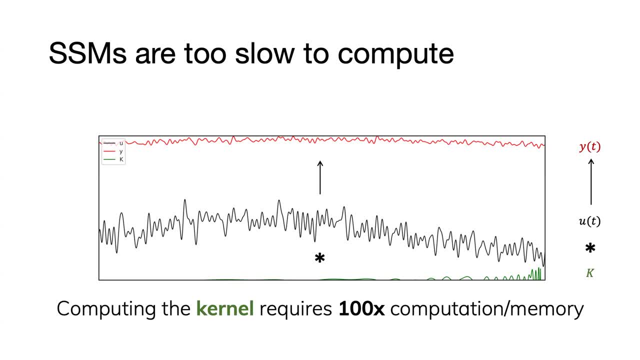 It was more of a proof-of-concept thing about the model, but computationally it was incredibly expensive and not really feasible in deep learning. But I guess, when you refer to it right, that we all have the same problem with just normal RNNs. 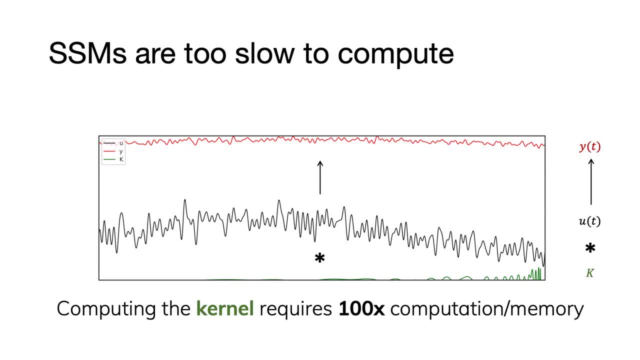 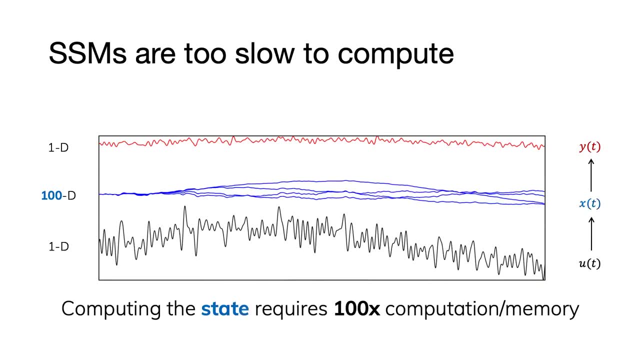 depending on the size of this even state right, Yeah, Yeah. so the reason this doesn't happen with normal RNNs is because they're defined a little bit differently. But here the main thing is that these SSMs, they kind of have a hidden state. 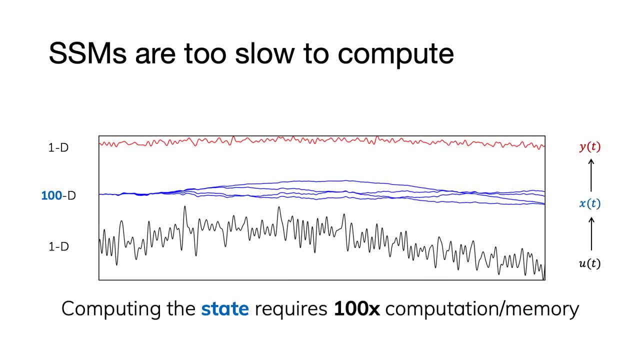 that's much bigger than the size of the input. So normally in RNNs, like you have an input of size like 1,000, and then you mix them and then your hidden state also has size 1,000. But here, if you have an input of size 1,000,. 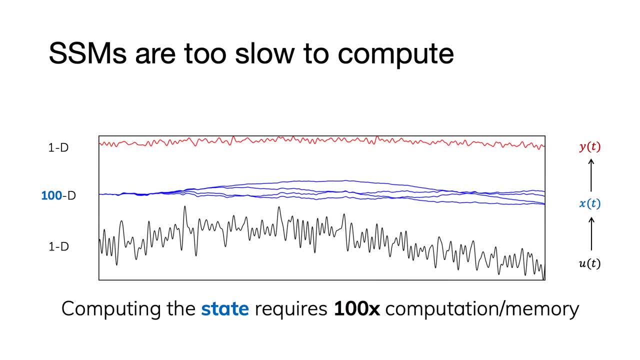 your state will be 100 times 1,000. So it's going to be very massive, Yeah, so that's kind of one of the main differences between the ways these are defined and RNNs are defined. It's like it's very reasonable to call. 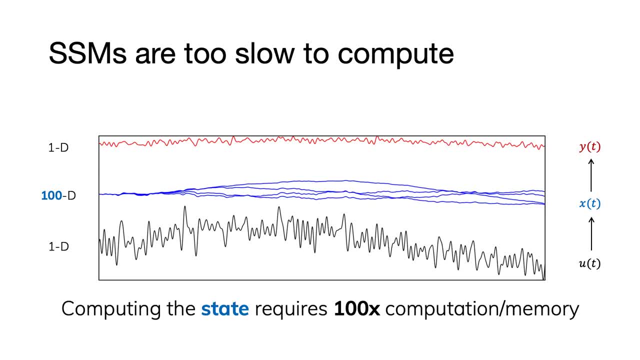 like SSMs. a theme is that we've been over is that they are RNNs and they are CNNs, And so various people will insist that they're RNNs or insist that they're CNNs, and that's true. 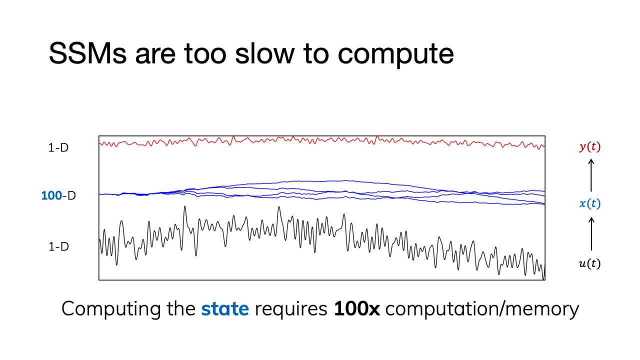 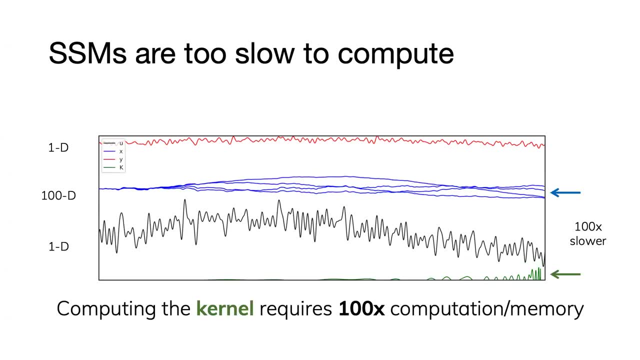 But they also have these extra properties where it's useful to have. you know, distinguish this intersection, SSM, Right. so where were we? Yeah, yeah. so these models? basically, this is one reason why I think actually they were- they're never used in deep learning. 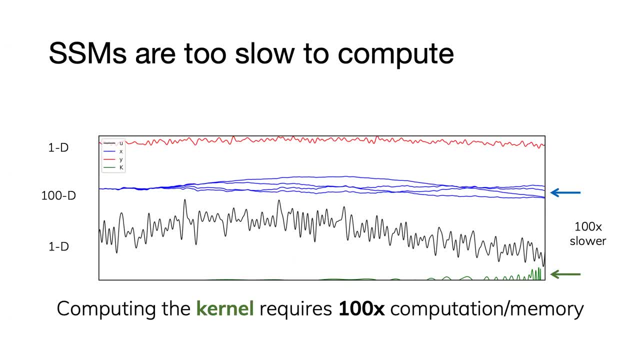 even though they've been around in other scientific fields for a really long time. One thing is just because of the different perspective, from statistical to deep learning perspective. Another one is that they're really impractical to compute in deep learning. So now the whole insight of S4. 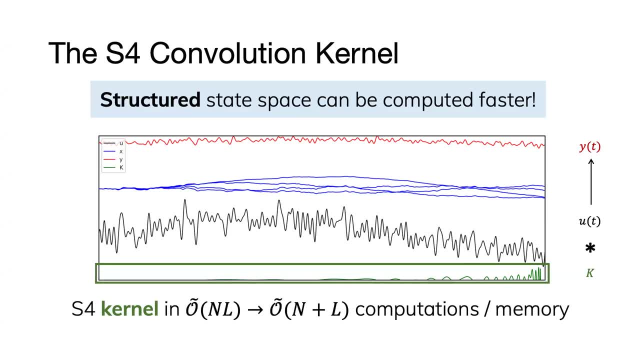 or the structure state space sequence model is that in order to overcome this, you need to impose structure on your matrices or structure on your Ssms, And then you can compute this whole map faster. So I mentioned the computation and the time and space complexity was n times. 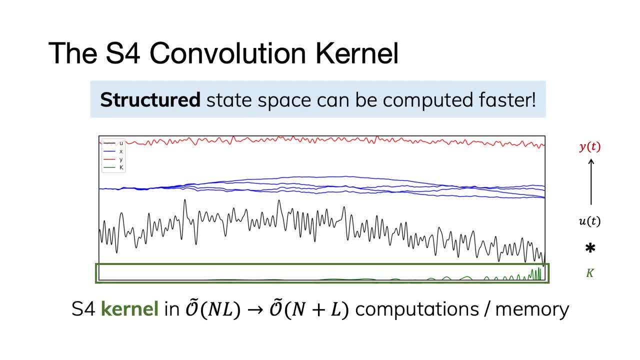 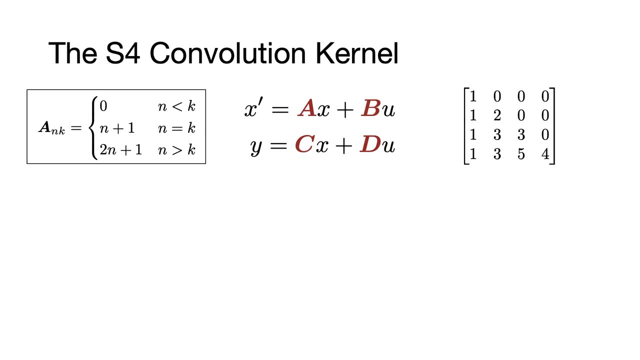 L, where n is the flow up into the state dimension, and you can reduce this down to a linear, which is a really massive saving. So this is what made it kind of practical to actually use. So the algorithm, it is pretty complicated and there's simplifications later. 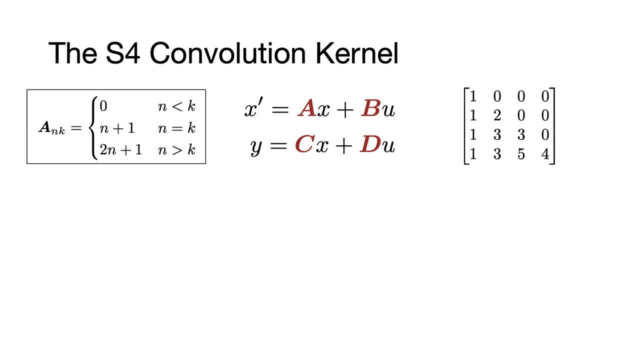 So no one really has to look at it, hopefully. But the idea is that again we have this SSM here. We are using fixed formulas for it. You can see that these formulas are highly structured in certain ways, And you have to figure out the right structure. 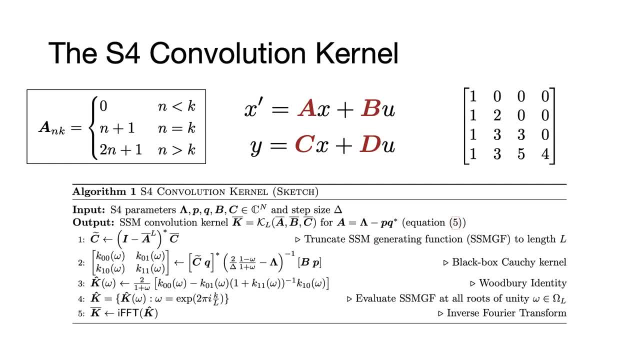 to look at it with And then with a specific structure. I found a way to compute this really efficiently using this pretty complicated algorithm. But yeah, this was kind of the main point of the original S4 paper actually was just like: how do you compute this thing as reasonably? 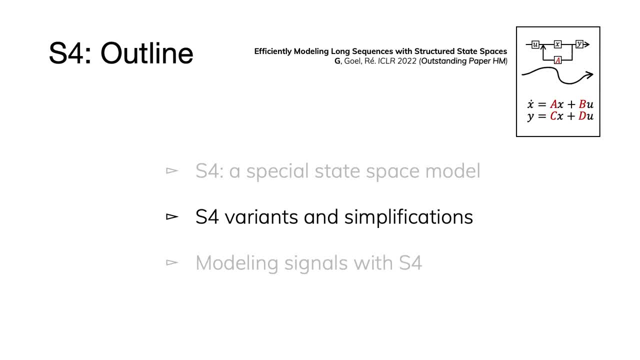 So there has been a lot of work following it. that simplifies that a lot, And these are the ones that I think are quite practical and a lot easier to use. So these are what is more commonly used in practice nowadays, So I'll just briefly mention some of those. 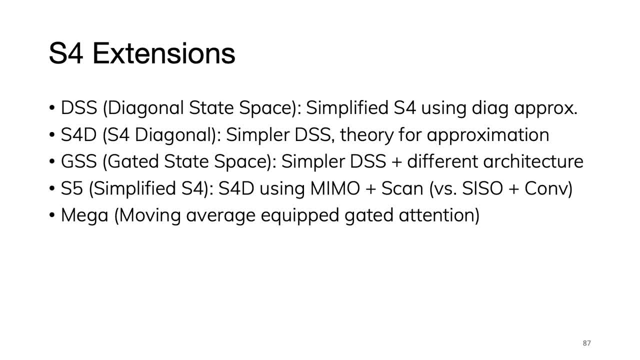 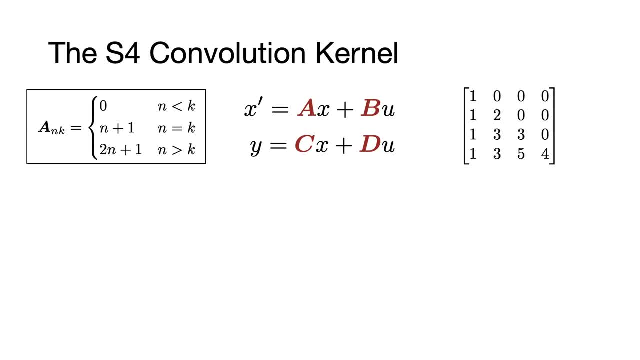 Essentially, all of them are Based on diagonal matrices instead, So I didn't actually quite define the structure I used here, But you can kind of transform this matrix into something that's close to a diagonal matrix but not quite diagonal, for various reasons. 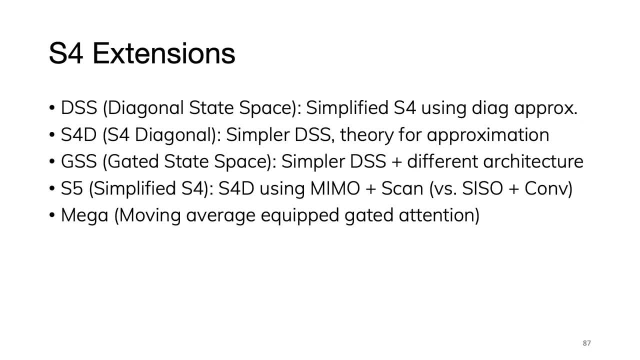 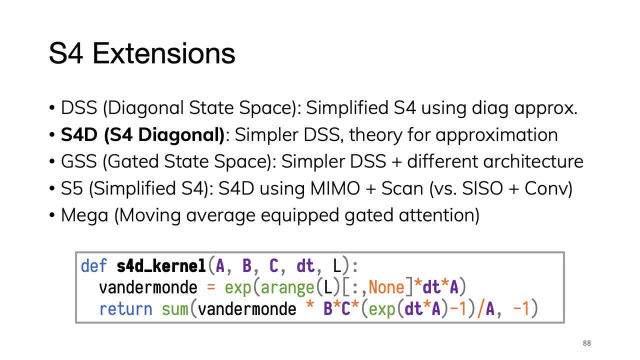 But later on it was found that ways to simplify it further into a diagonal matrix, And so the official one, like the basic version of this, is called S4D, which is just a diagonal version of S4. And And that very complicated algorithm from before. 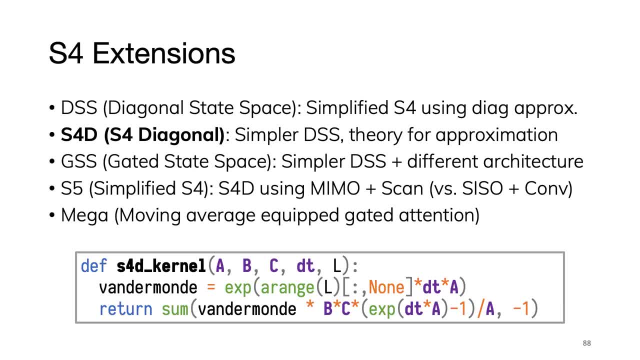 which was for computing. the convolution kernel can be simplified down to just a couple lines of code. So this box just is: how do you? I mentioned, in order to use the CNN mode, you have to compute the convolution kernel, And that can be non-trivial. 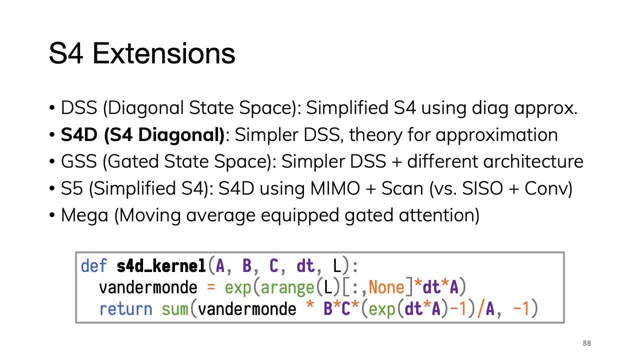 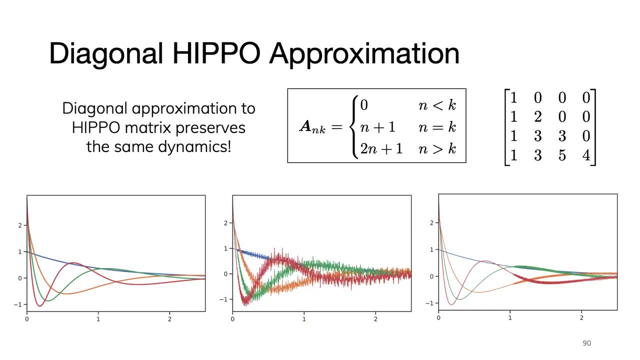 But for diagonal matrices it's quite simple And you can do it in two lines of code. Technically, one of the things that made this hard was: can you define these diagonal matrices while also having nice properties? Because in early versions of all of this, 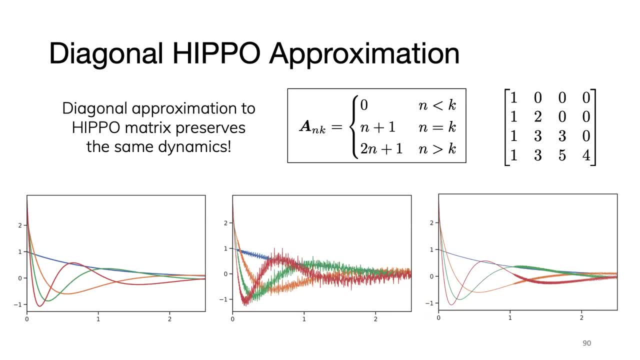 basically, I also found that a natural question is: do you need HIPPO in all of that? What happens if you just have, say, a random state-space model, And it turned out to be quite hard to find the ones that worked? 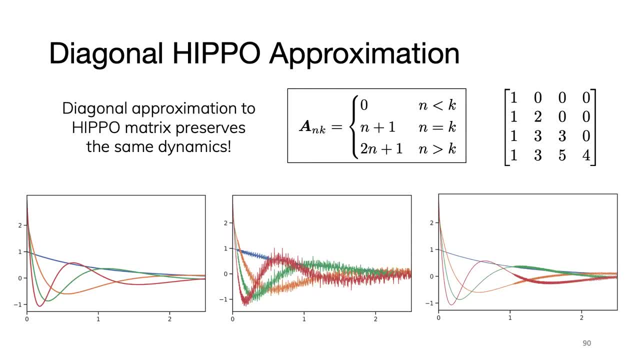 So actually it seemed like the HIPPO theory was actually quite important, And if you just make a random SSM or a random diagonal SSM, it doesn't really work that well. And so one of the insights needed to make the first diagonal one work: 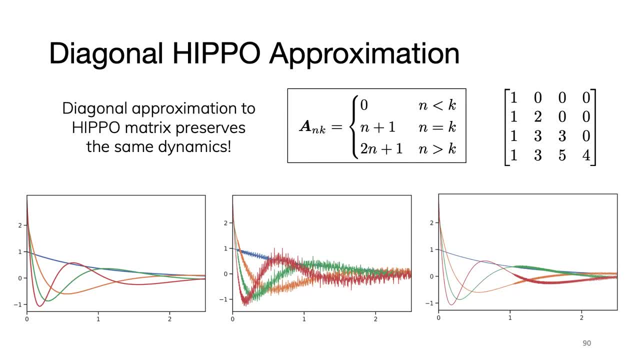 was discovering that there is a. it's actually very surprising that there is a diagonal approximation to this thing that basically has the same dynamics. I don't really have time to illustrate this, But you can view the convolution kernel as some set of basis functions. 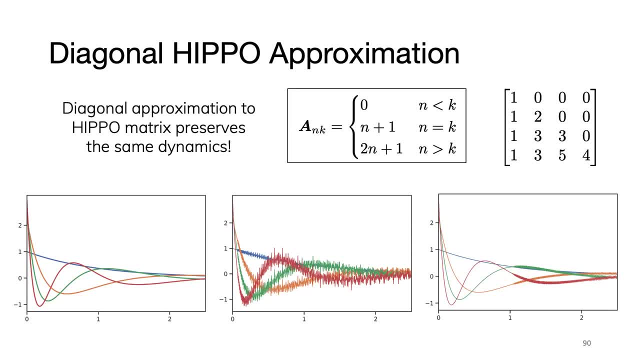 This is the one for HIPPO or S4. And by using a particular diagonal approximation you get these fuzzy approximations of the same kernels. So again, this is actually a really surprising fact. actually, Even now, to me it's still surprising. 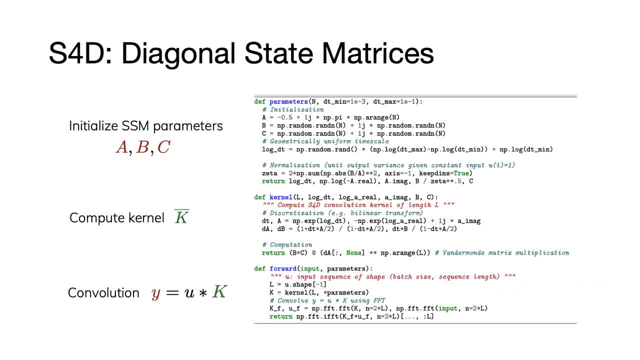 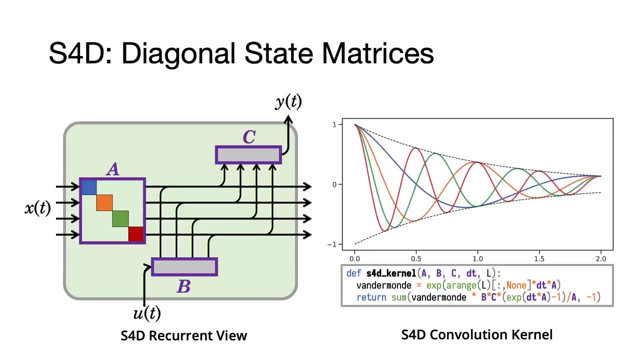 Yeah, and then computing the whole thing is very easy. So this is like an entire self-contained code sample of initializing and computing the entire forward pass of the model. This is all available online. This is kind of like Another way to view it. 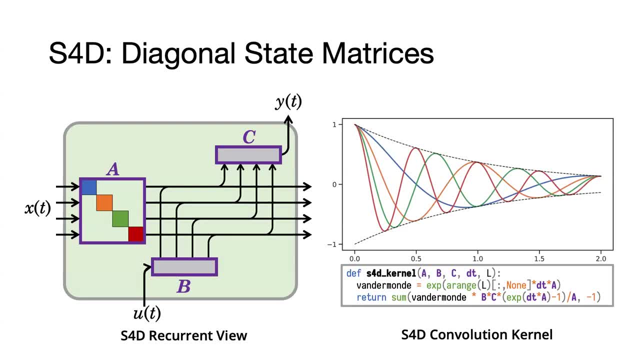 As an RNN, you have this diagonal A matrix And when you're, if you think of an RNN and you're multiplying by this A matrix, if it's diagonal, then essentially every single channel or feature is operating completely independently. Because when you multiply by diagonal matrix, 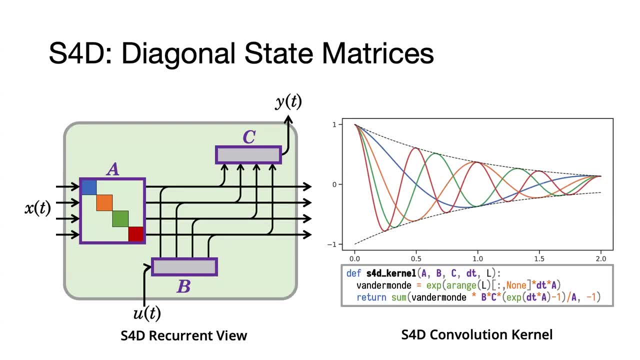 it's just a scalar multiplication, element-wise multiplication. So if you drew an RNN cell for this- which is people like drawing LSTM cells and stuff- it would kind of look like this, where every single channel is actually operating independently, which is one reason why it's very simple. 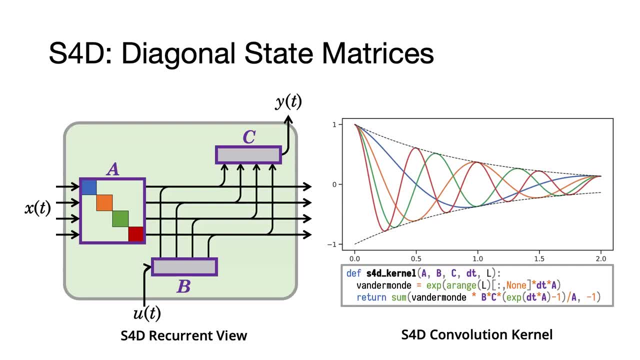 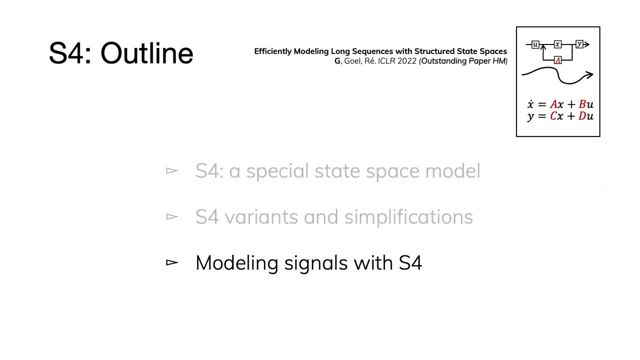 And as a convolutional model. there's other interpretations for it that are also pretty simple. OK, any questions about this? OK, so I think in the meantime we can look at a couple of experiments for fun, And these are actually some of the older experiments. 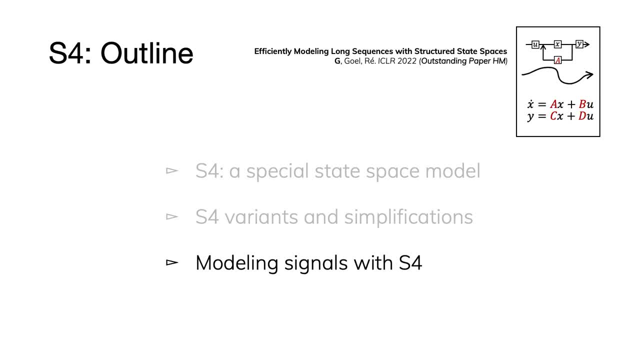 And there's been a bunch of follow-up work and a lot of other interesting stuff, But hopefully I have all the good ones, Yeah, so one thing, as I mentioned to emphasize is that S4 was known for two, the thing it was originally. 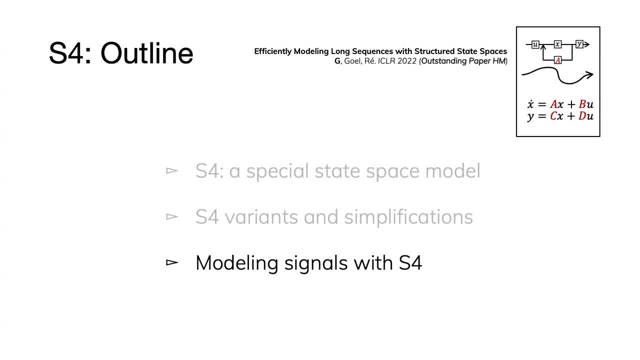 known for was for modeling long sequences, which was one of the motivations through Hippo, But actually I think that one of the main strengths is not necessarily long sequences, but it's about sequences that are continuous, which I alluded to at the very beginning. 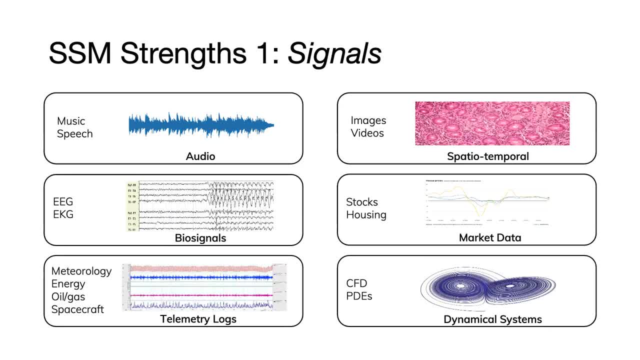 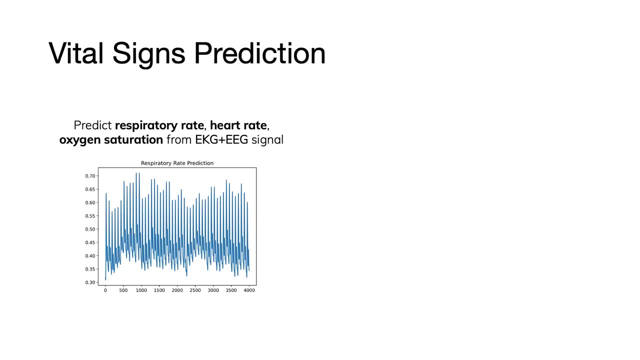 So you can call this signal data, which appears a lot So, like audio waveforms, images and videos, any sorts of time series. there's lots of this type of data in the world, So here's an example. This was a classic time series benchmark. 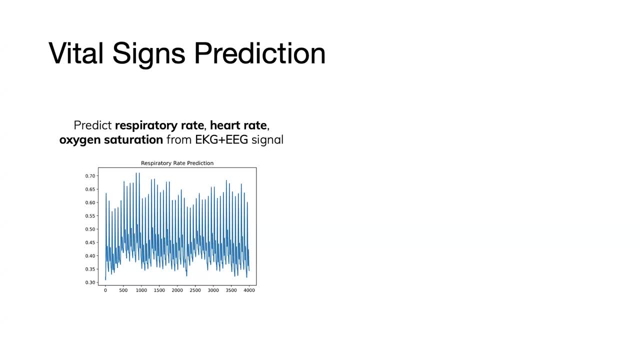 where the input data was these biosignals like EKG and EEG and PPG, I think, And now, given one of these input time series, the goal was to predict the patient's average heart rate or respiratory rate, like a couple of these biometrics. 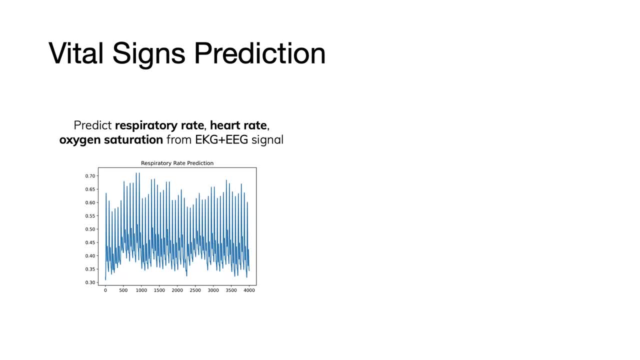 So, if you look at this, so this particular data was challenging because the inputs were length: 4,000.. Normally, for a long time, people had a hard time scaling things past even a couple hundred or 1,000. And this sort of data has very different characteristics. 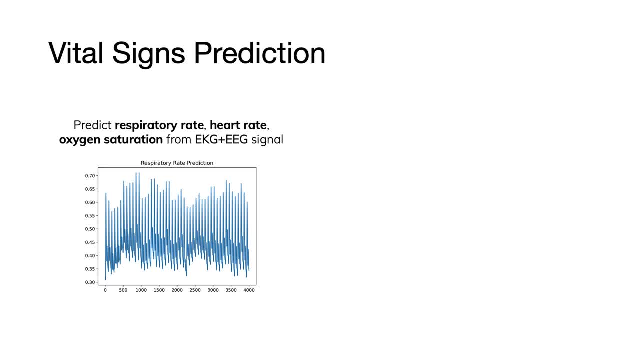 than data such as text data. If you visualize the signals, they look like this And you can see that there's very strong periodicity. That's a common feature of signals, If you like. when we zoom out like this, you can see that. 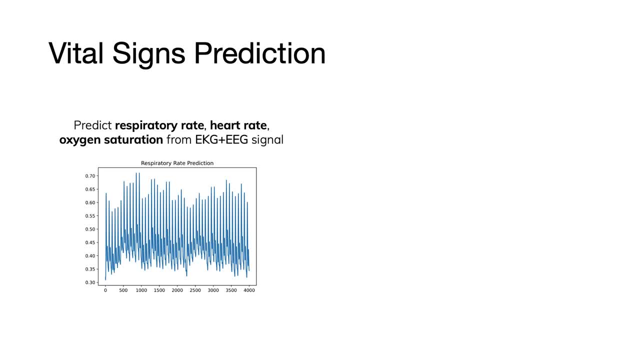 But if you zoomed in all the way, actually these signals are very smooth. So they're kind of because they're sampled at a high rate from an underlying continuous signal. So this is the exact Type of thing that these SSMs are really good at. 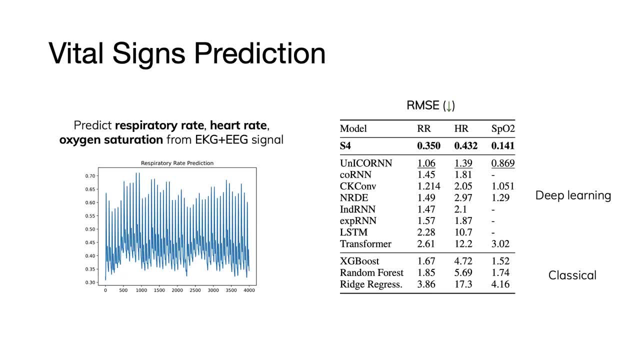 There was a couple of papers that did a bunch of benchmarks before this. I think my computer might run out of power soon. We'll have more. OK, Yeah, so this is a table of results for just regression on this time series. We're just trying to get as close as possible. 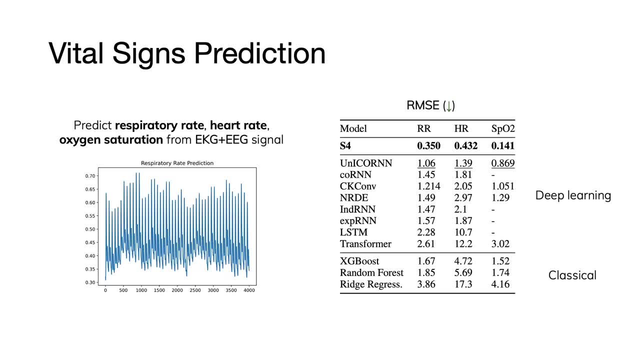 to predicting the patient's heart rate or something, And there's lots of baselines here, including more classical ML approaches like boosting methods and forest and so on, and then a bunch of deep learning sequence models such as these RNNs and CNNs. 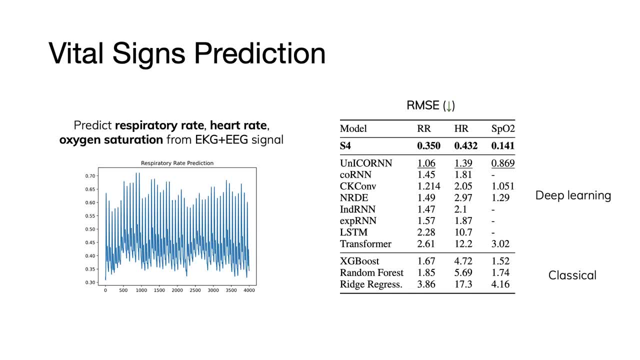 And as far as just much better than all the baselines here. One thing that I think is interesting to point out- and this is just one example- is that, coming back to this question of inductive bias, I think that people throw transformers at everything nowadays. It's supposed to be like a magic pill, but they're actually. 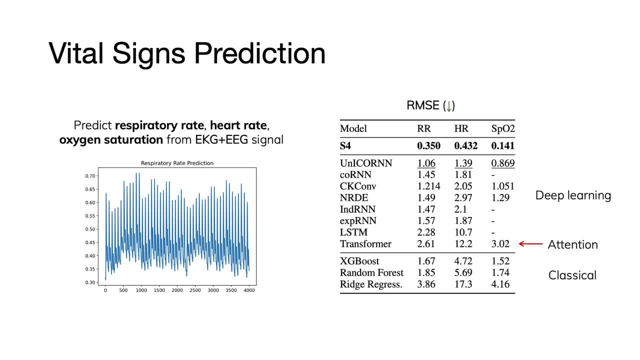 I think they're very, very good at modeling some types of data, but they don't have the right inductive bias for other types of data like this. So if you just threw a transformer at this sort of very smooth, very long data, it really struggles, and other similar things too. 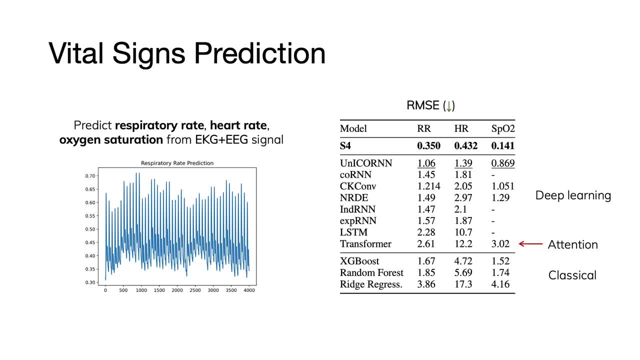 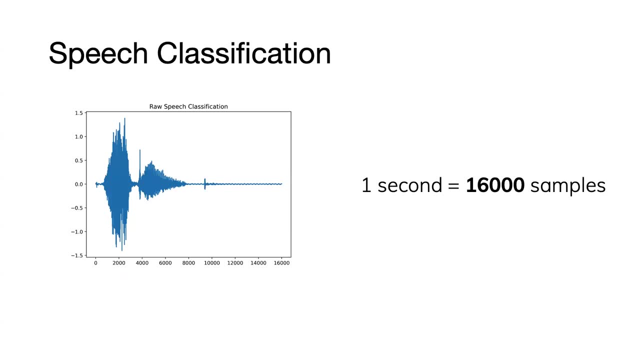 There's lots of places where you basically need to have a CNN encoder or something like that before you can feed it to a transformer, because it's not going to work on the raw continuous signals like this. Okay, and now we can sort of see some of the properties at work. 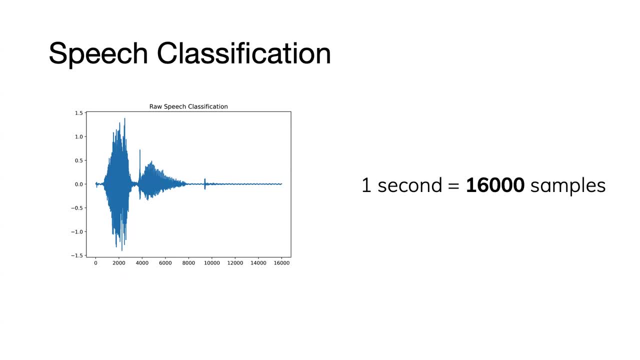 on the data. So I'm going to go ahead and show you some of the properties at work More specifically. so here's another example of a signal, which is speech flow classification. So, again, audio waveforms are continuous and they're sampled at an extremely high rate. 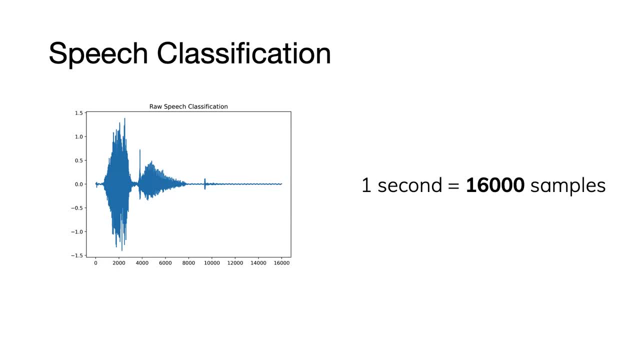 like 16,000 hertz or even higher, And this is a data set where you get these one-second speech clips, which is 1D sequence of like 16,000.. You pass it through a deep network and you're just. 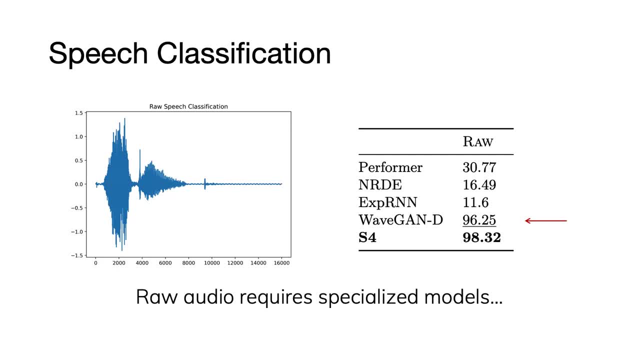 trying to classify which word was spoken in this waveform. So, first of all, because the sequence is so long and other problems: lots of models don't work well. So RNNs and these transformers, and I mean a vanilla transformer, won't even work here, because 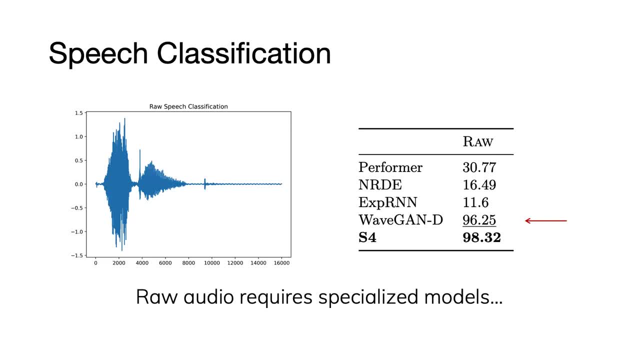 the sequence is too long. But there's these transformer- approximate transformers. They don't work, RNNs don't work And other neural OB-based methods don't work. CNNs do work here And because SSMs are CNNs, they also work very well. But I think what's a lot more interesting- 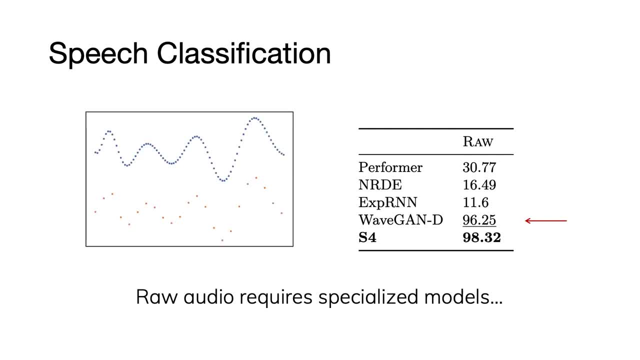 in this setting is- you can ask the question that. so audio is sampled from an underlying continuous waveform right Now, if you sample it at different rates, you're still getting the same. it's still the same underlying signal And it's still the same word that's being spoken. 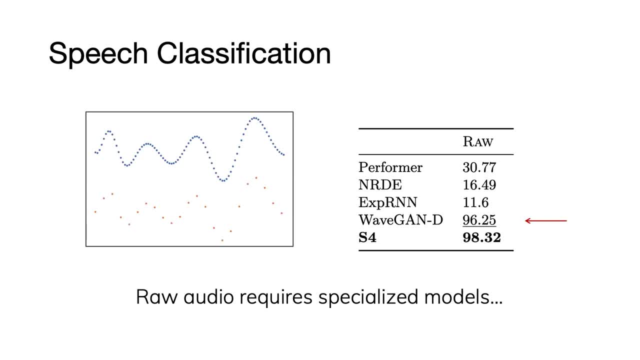 But if you fed in this blue signal sampled at a certain rate, versus the orange signal sampled at a different rate to the model, they might look very, very different. And so, in fact, if you look at CNNs like normal local CNNs, they will completely break if you train them on one resolution and 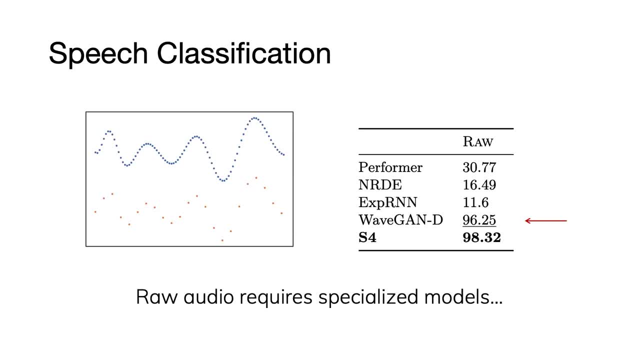 tested them on another resolution, because the convolution kernel is kind of very attuned to exact. If you have convolution kernels with three adjacent things on the blue signal it would look very different than three adjacent things on the blue signal, And so if you do this, zero-shot frequency change is one word that we called it. 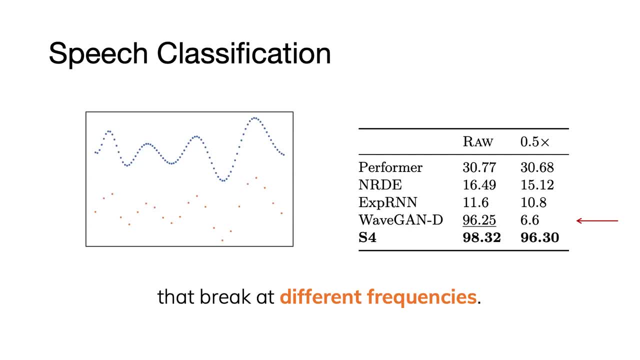 the CNN baseline that worked well, just doesn't work here at all. unsurprisingly, But because SSMs are a continuous model. this is one example of a concrete empirical benefit that you can get from it. What happens here is at test time, without training, at a different resolution, you can just: 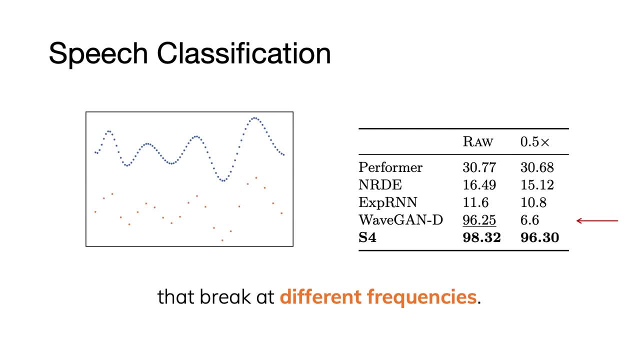 change that discretization step size. So remember, there's like this extra delta parameter I mentioned. It kind of represents the spacing between the things And so if you train it on one, then if you're testing it at a different resolution, you just scale the delta. 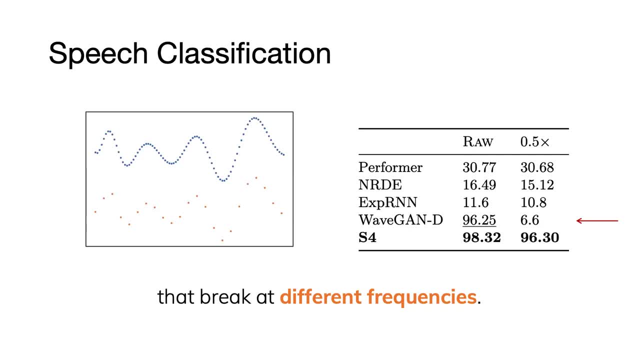 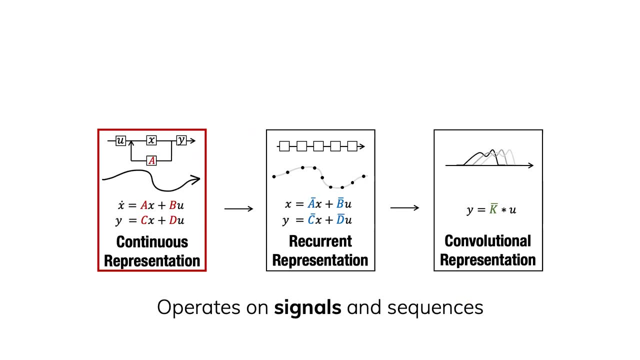 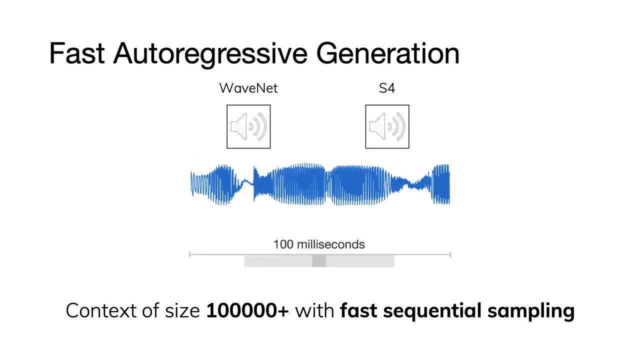 appropriately and it will just work out of the box. So this was the point of the continuous view. Now, what about the recurrent view? I've kind of gone over this about. it's very good at auto-aggressive, but it's also very good at auto-aggressive settings. So an example is you might have heard of. 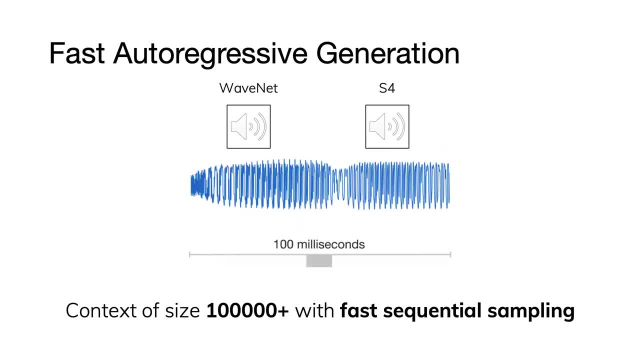 WaveNet, which was the first model to be able to do a raw speech generation. It was the first like speech-generated model. And these were all auto-aggressive models where you take it, you just sample like this, one sample at a time, And there's a lot of challenges because you can. 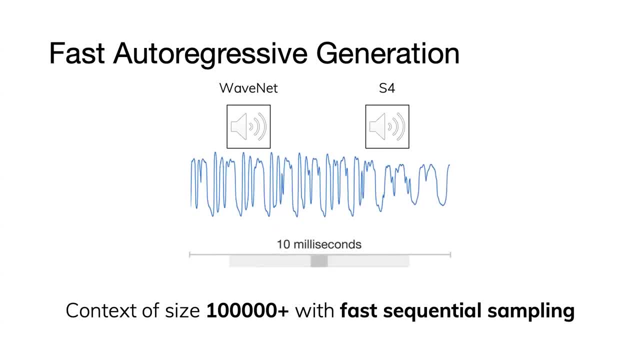 see that the audio signals look very different at various resolutions. They're very smooth when you zoom in. they're very important, they're very periodic, and so on, when you zoom out And yeah, so it's hard to model and it's also hard to sample. 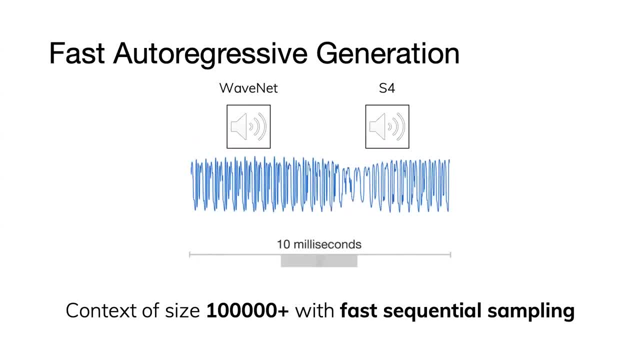 fast So you can throw in an SSM and it gets this unbounded context that we talked about. So you can have a huge context but still sample very efficiently, because it's an RNN that has a finite state size And WaveNet has actually been. even though it's been, it was like, like 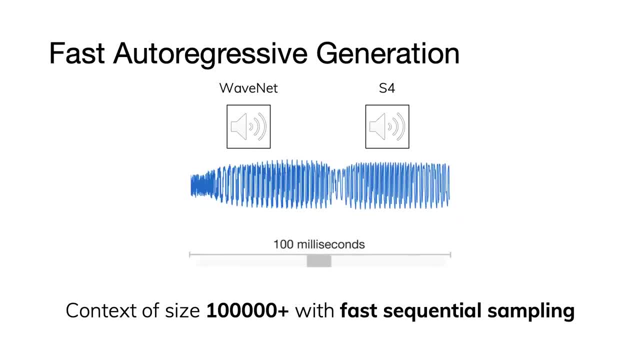 2016 or something, it's still actually the best auto-aggressive speech model based on these like value convolutions and so on. Well, so auto-aggressive speech sampling isn't that popular nowadays because of other. there's other approaches, but if you were to do, 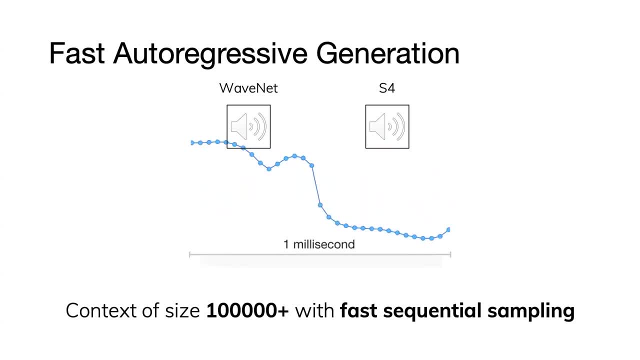 auto-aggression. WaveNet is still the best And we try training it on this particular dataset of speech where, basically, these one second clips of people saying English digits like 0,, 1,, 2,, 3. And WaveNet just didn't really work at all. I think there might be a demo here, but 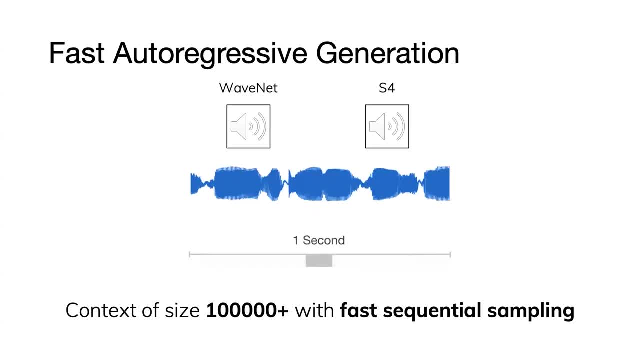 I'm not sure if my volume is on. Yeah, I'm trying to see. Okay, Let me, let me try this. So here's a WaveNet sample. It's basically just garbage. And then here's the S4 sample. it's trained in the same way. 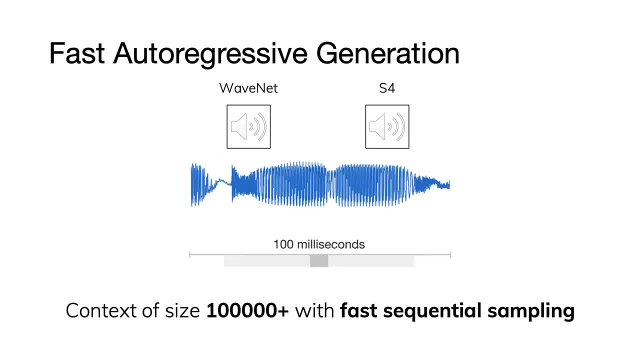 1,, 2,, 3,, 4,, 5, 6.. So it's a it's night and day here. So this is one example of something that kind of. actually it leverages all of the properties. So the way you do this is that. 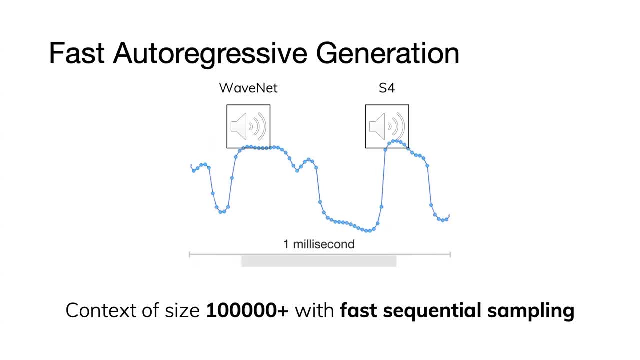 during training time you get this, you get a very. you've got this sequence and you're doing auto-aggressive prediction of the next one, while during training time you do it across all time steps at the same time. So you need to be parallel and you use the convolutional mode to train And 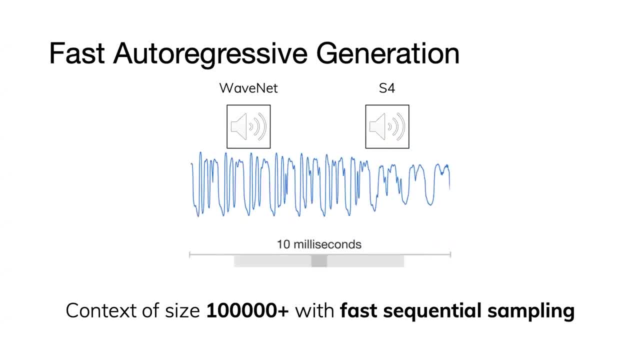 then at inference time you switch it into the recurrent mode, which generates things in a very much faster. And the continuation. it's an old version of the training and it's just yor. So one of the things that you got is to: you know, if I want to train an example of an 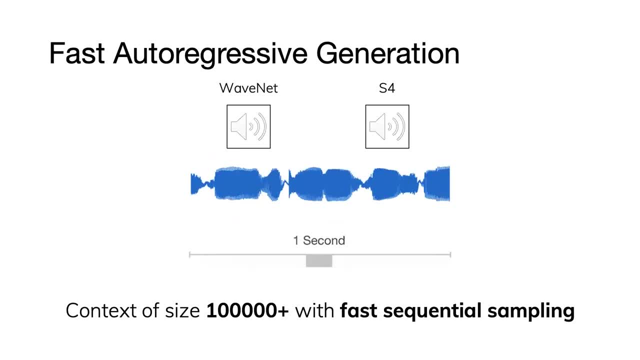 auto-aggressive prediction of the next one. then you have to think about: am I going to do this? If I can employ the interval, it's going to be a little bit faster. I'm not going to be in an um and the continuous one is more fuzzy here, but it's just the reason. like those are all about the. 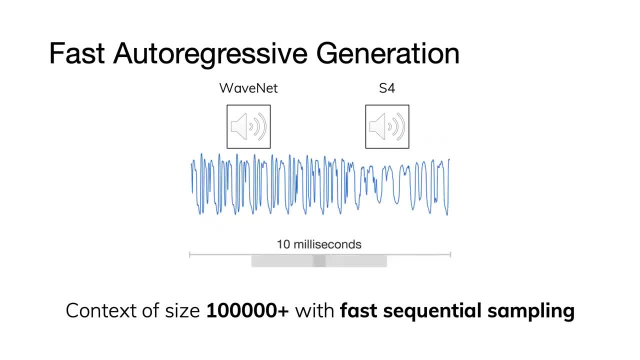 computational properties like the rnn and cnn modes are about computation. but why is it actually modeling like? why does it sound so much better than wave net? um, that can just be contributed to the inductive bias of being having the right bias for modeling these types of continuous 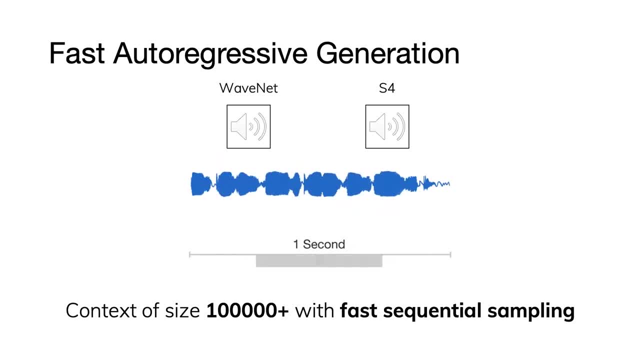 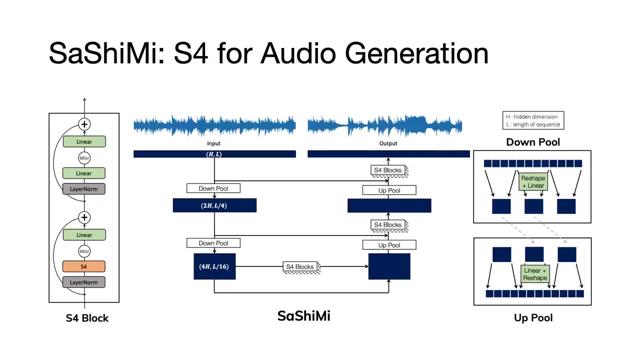 signals and being able to get lots of context into the model. um, but yeah, i usually use this to illustrate the recurrent view. um, yeah, this is all. yeah, this is a model called sashimi. i uh, basically it's just using s4 as a black box into a different deep neural network architecture. 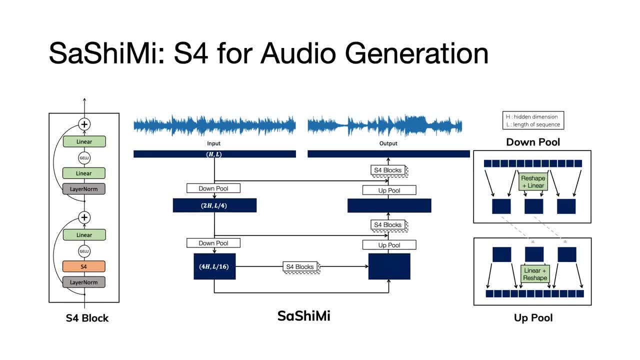 um, and one thing i always emphasize is that um, ssms and s4 are not a deep neural network. so i mentioned this at the beginning but just to reiterate, um, i think of them kind of as like a primitive building block. that's just a simple linear sequence of sequence transformation and 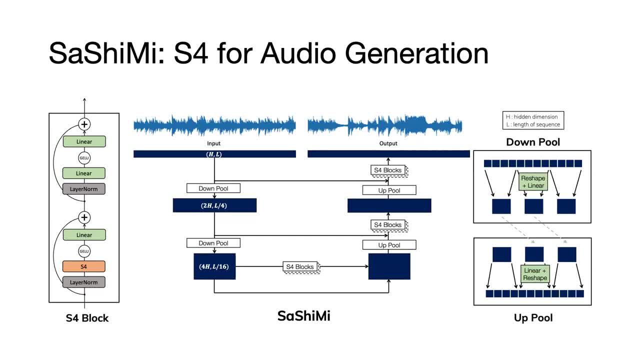 you can incorporate them into your neural network, and then you can incorporate them into your neural network, and then you can incorporate them into your neural network, into deep neural networks in lots of ways, just like you can incorporate, like uh, convolution into a deep neural network in many ways. um so, this sashimi was a particular. 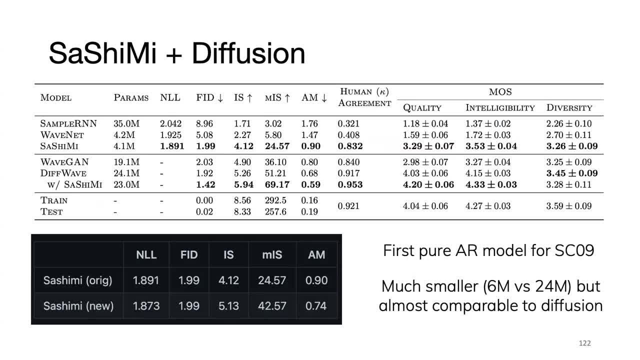 architecture and you can also use it in different settings. it doesn't have to be auto-aggressive um. you can use it in diffusion models too, where, uh, by replacing the architecture in a diffusion model um with uh something based on s4, it also improves that model. 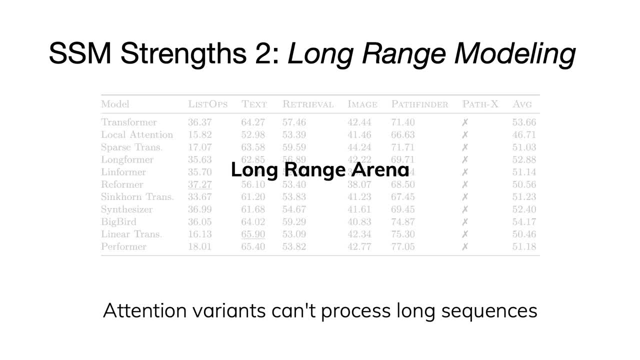 um, okay, i think that's pretty much everything. um, i guess the i just mentioned the one, the thing that s4 was originally known for, was, uh, modeling language dependencies and um, attention was famously famously struggles with this, which is part of why lots of variants have come out. uh. 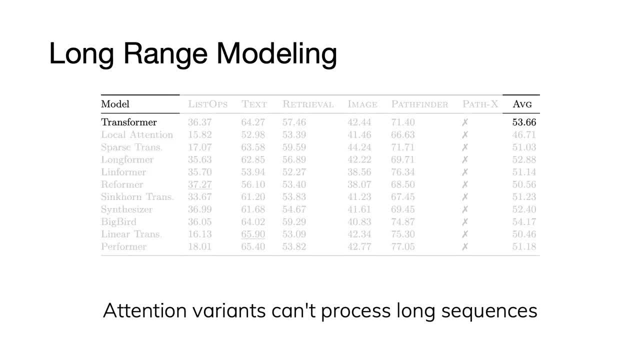 that are supposed to be better. um, but there was this benchmark called language arena. that, uh, gave a suite of six tasks that were pretty hard for and they had sequences of length a thousand to 16 000.. it was pretty hard and all the transformer variants were about the same, which was not very. 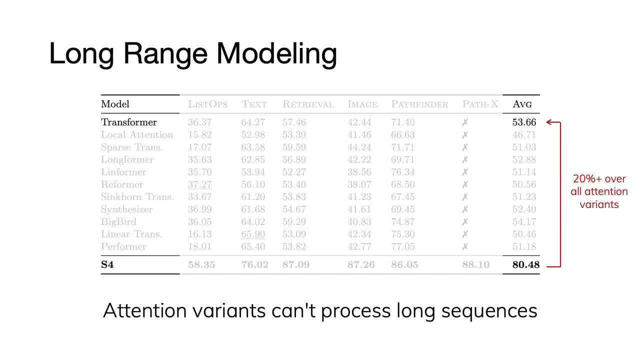 good, um, and when s4 came out, it improved the state of the art here by over 30 points. uh, actually this, this is an outdated number, um, but uh yeah, so it was kind of known originally for doing being able to do this long-range modeling, um, as well as solving some very, very difficult tasks that. 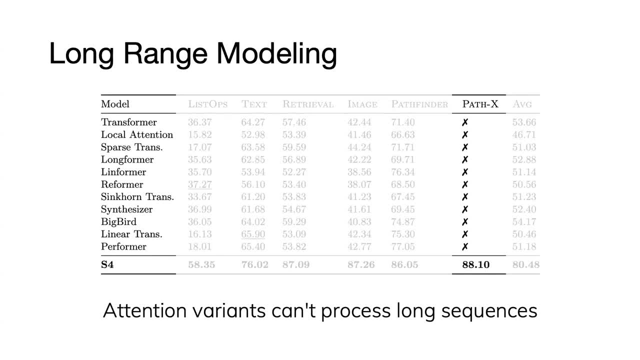 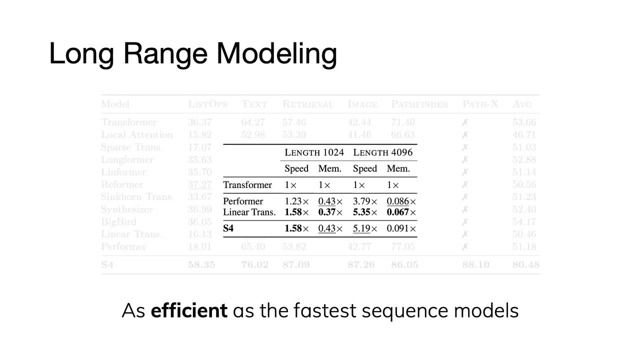 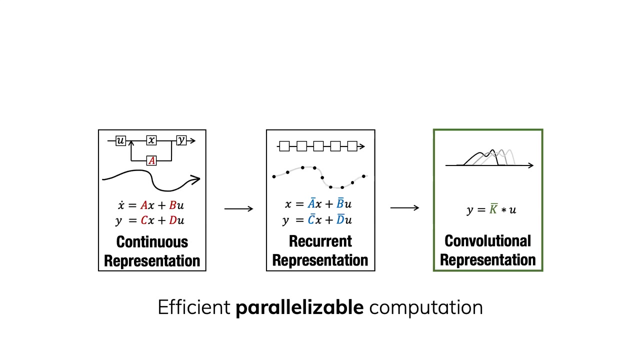 uh, no, transformer can even achieve better than the man guessing app. um, yeah, and then there was also benchmark kind of the speed of these different models against each other, where, um, because of the the special fast algorithm that i mentioned, uh, it's also, basically it can be much faster than transformers, especially as the sequence gets long. okay, um, i. 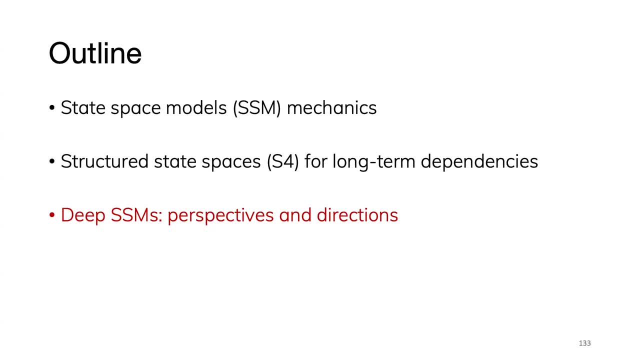 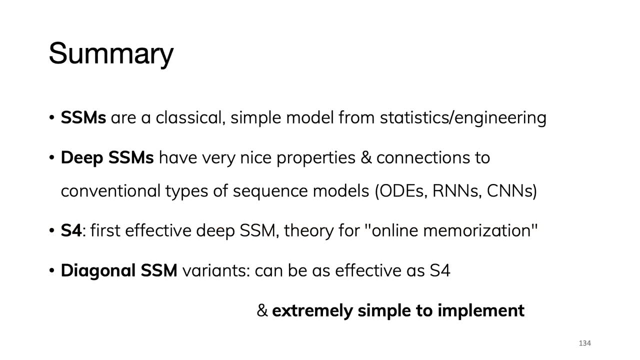 think that's all the time i had. there's some other stuff here about comparing like ssms versus other models. um, that's not that important, so well, okay, here's actually one summary slide. so, um, yeah, so safe based models, old model, but uh, different use in their classical statistical 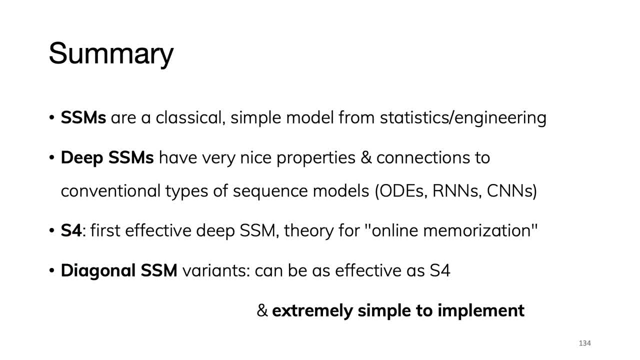 sense than what we use um in deep learning. we think of them as having lots of computational benefits, um, and they kind of generalize or are very related to lots of classical sequence models like rns and cnn's um s4 was the first deep or structured ssm. 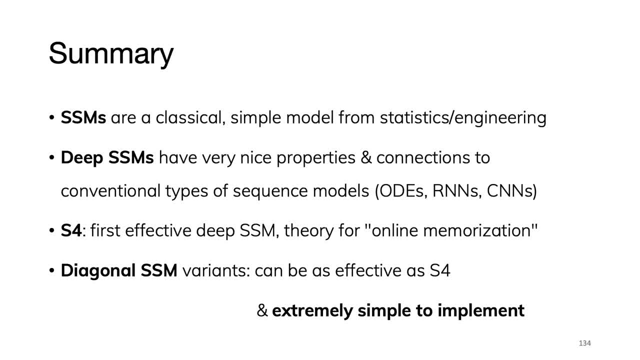 and um. it was based on the hippo theory for this online function- reconstruction or online memorization, um, and in practice, i recommend people to use the follow-up diagonal variants, which can be empirically as effective but can be a much simpler to implement. um and if you email me, i can. 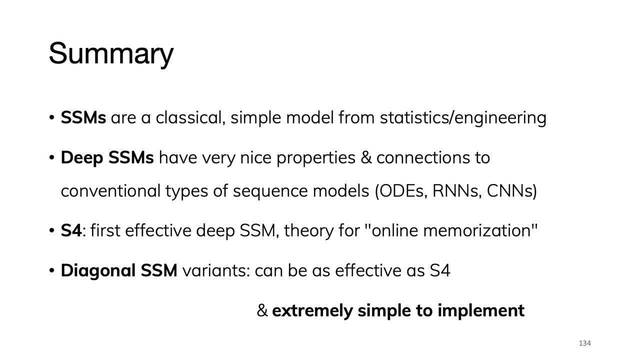 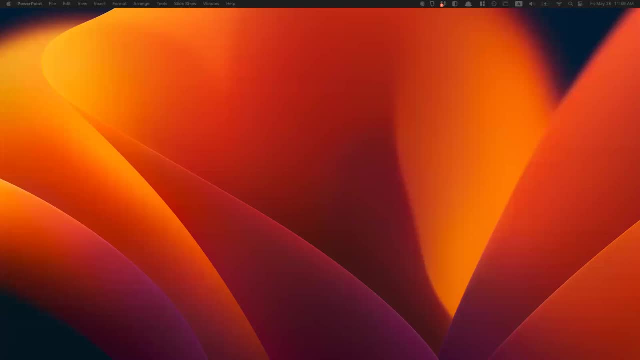 send you some resources in blog posts. actually, i'm currently writing up a um well, i procrastinated on my thesis for a year and i'm finishing it up, which will also be a general tutorial on ssms. yeah, that's everything. uh, any more questions? okay, so we've had time for a few questions, maybe. so, while we are coming up with your questions, 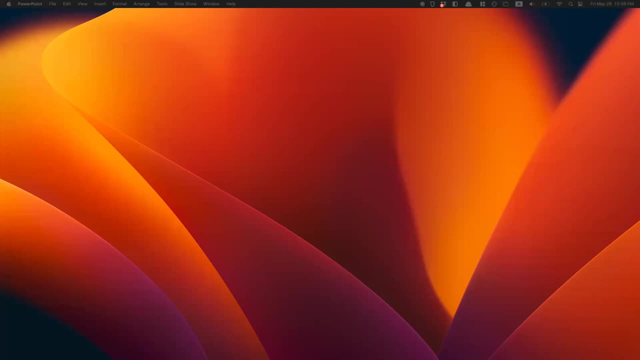 like there's already one question online so i'll just read out to you. sure, okay. so uh, colleagues asked: since s4 has some close connections to vanilla ins- vanilla is okay- how do you overcome gradient exploding or vanishing- issues that arise to long-term modeling? yeah, great question, so um. 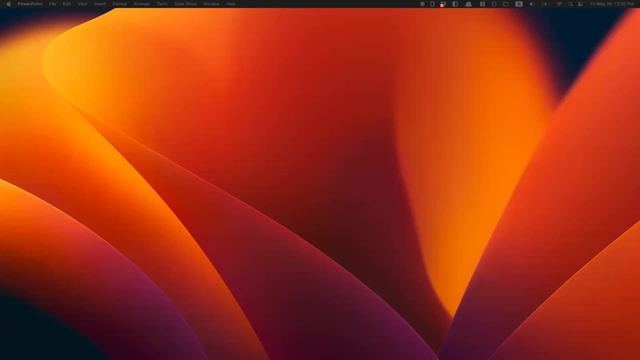 there's a number of perspectives on this. um, one way to look at it is so you can look at it mechanically. you can look at it kind of like at a higher level. um, one the higher level answer is that, uh, when you use something like hippo- um, hippo was designed for. 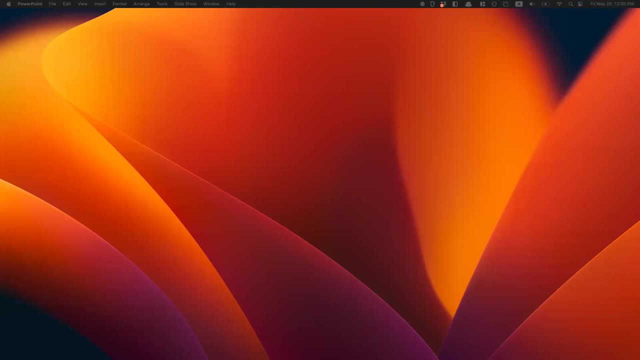 this long-range memory and uh, it's basically constructed in a way that, by definition, avoids um vanishing gradients. i mean, another way to look at it is that, uh, hippo is designed to like to remember all this history and um, essentially, that forces it to not have managing uh gradients. um. 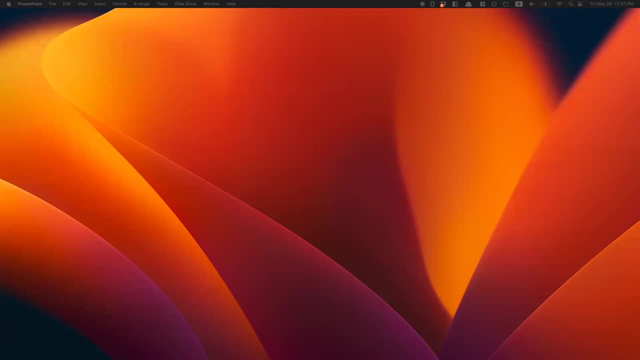 or like its dynamics don't decay through time. but that's that may be not very satisfying um, you can also look at the very mechanically. which is that? um, if you look at the. so one reason why it's this is better than normal rnns is because of the fact that it's linear, and when it's linear you get control over. 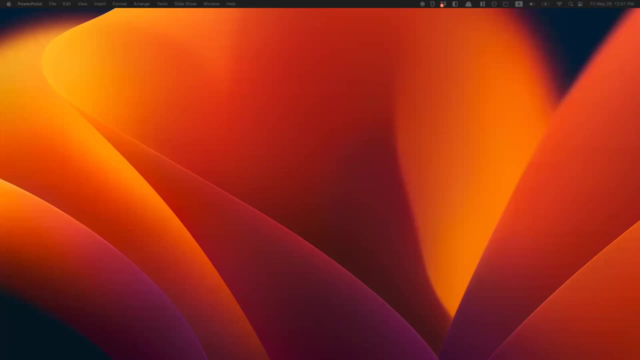 the dynamics. you can control the dynamics of the model much more precisely. um and in particular, for example, if you look at that a matrix, that or the, a bar matrix that you're powering up, if you can control the eigenvalues of that matrix, then you know exactly how fast your uh, your, your. 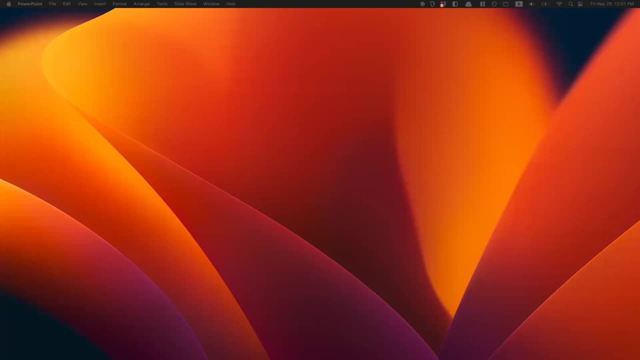 like signal vanishes through time, um, and so basically, yeah, you can, you can constrain it in a way to make sure that it will have. it will vanish exactly like it will. it will capture dependencies for exactly as long as you want, um, and when you plug in the hippo matrix, it sort of 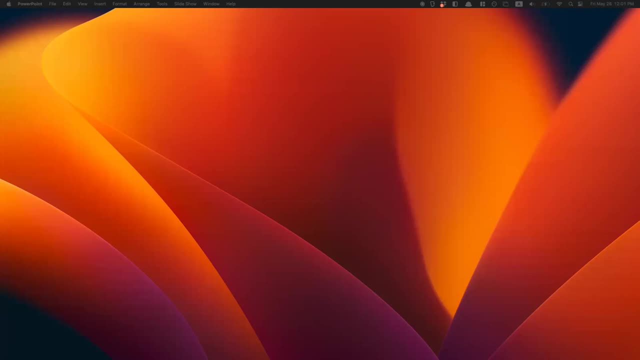 does that by default, um, through other interpretations, but uh, even without that, there's many ways to make sure that it's um not vanishing. yeah, oh, thanks, so you're on the question. yeah, uh, yes, so this is a good question too. so, um, some people will point out that um. 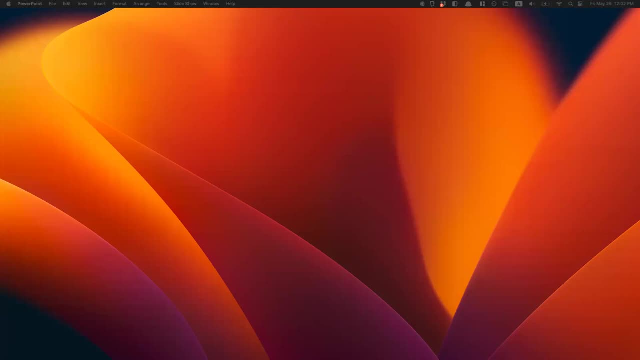 if you have. if you have a fixed model and you want to compute it, you don't need to continually recompute that convolution kernel. you only need to compute it once. um like, if you're able see if your parameters are fixed, then you can compute the kernel once and cache it. 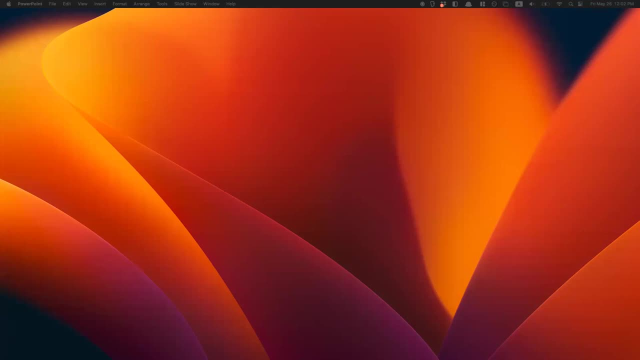 and then, during the forecast, all you need to do is the convolution part, which is actually cheap, um, but this only works after training, when you've already, like, trained your model's parameters and they're frozen. uh, during the training forward pass, your model's parameters are constantly changing. 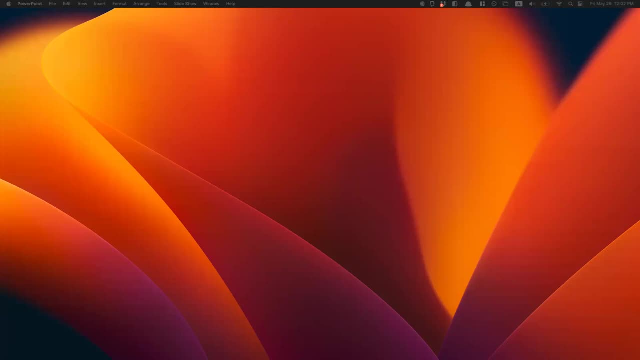 while you're doing great descent and you'll need to recompute that convolution kernel on every single mini batch, um, yeah so. so that's why it's very important to complete that kernel really fast, which was why, um, all those algorithms were developed. okay, so there's another online question. 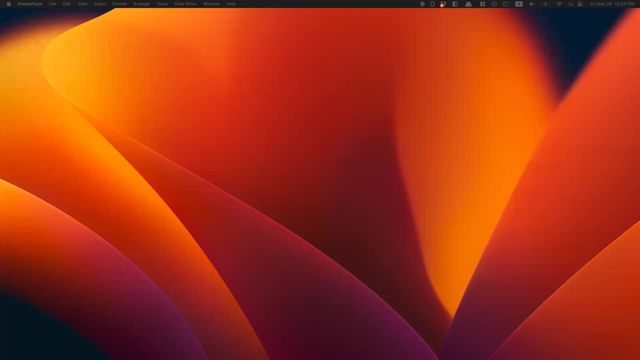 okay, so what's your perspective regarding the use of s4 um to graph structured data, for example, when connectivity structure between channels is not? yeah, so this is something that, um, i haven't really uh, worked on myself. there has been, um, there has been some work on this. there is. 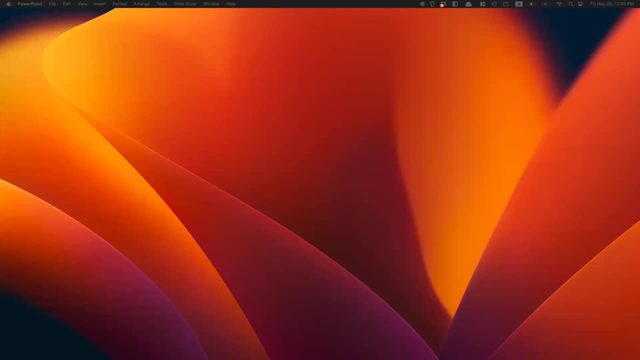 somebody in the stanford medical department who is working on eeg data, where you have like, let's say, like 20 channels, and these channels are all based on locations on your head, like electrodes, and so there's also this like spatial graph structure between them, and they found an extension by 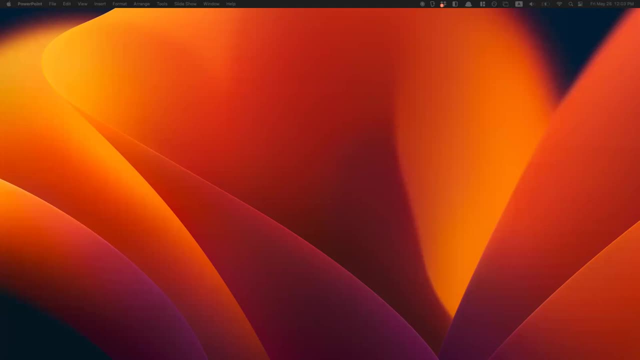 combining it with gnns. uh, that improves the model. um, i don't actually know the details of that, but you can combine this with other techniques, with gnns to to improve things. um, personally, i think in practice, especially in deep learning, there's, honestly, there's a lot of mystery about, like, how things work and why they work. but in practice, 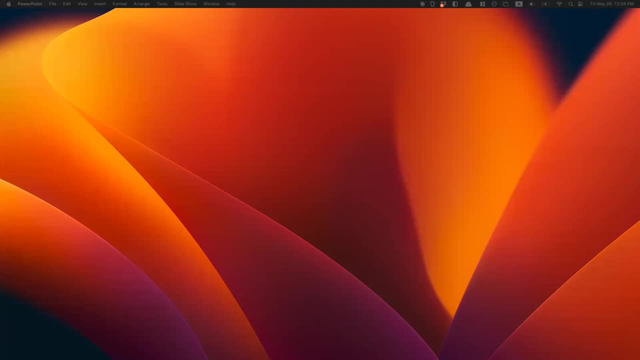 normally if you without baking in that structure, it works pretty well, just as you start scaling your models. um, that's the lesson people keep learning: just make your models bigger and you don't really need to bake in those structures. um, one thing i did i maybe didn't mention is that in the deep 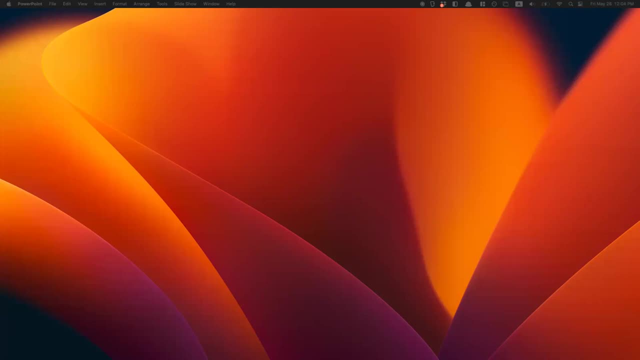 neural network architecture here, um, i kind of mentioned that if you have multi-channel data, you kind of um and i- i defined s4 as this- like one need to one d map, right? so what happens if you have multiple channels in your input? uh, you basically just find. 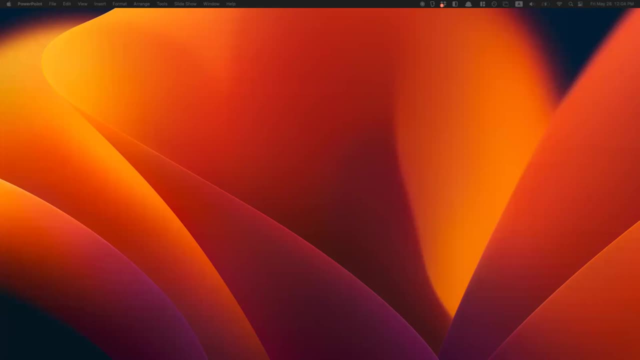 an independent ssm per channel and they operate completely independently, um. and but then after you do that, then you'll need to mix the channels in a way using like linear layers, mlps, or perhaps you can use some other like gnn or other structures to mix them. so that's kind of a flexible uh. 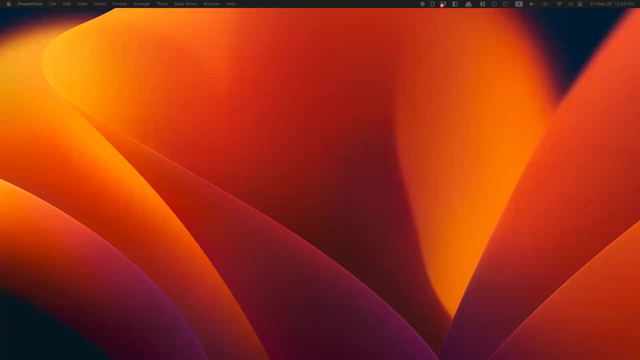 something, something else that's orthogonal to the main ssm part, so it's essentially like one ss, uh, s4 layer for the time, uh, more than another, let's say, of mixing layers. yeah, combined signals. yeah, exactly, and then you can start these two things. yeah, yeah, and then you just make it deeper and and it works usually okay. another question online. 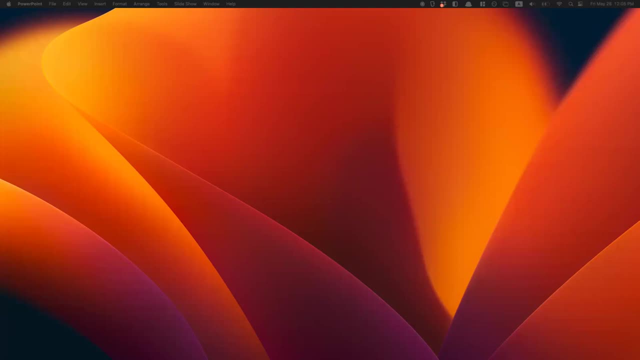 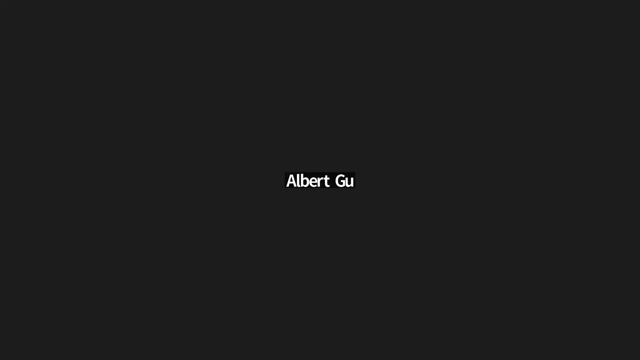 so in the context of online learning, are ssms, uh, ssm based deep models, more promising than other irons and transformers? um? so i think it depends on exactly the setting, but i think that i do think that online learning is one of the most interesting application areas for this um. so so one question is kind of like: in general, recurrent models have 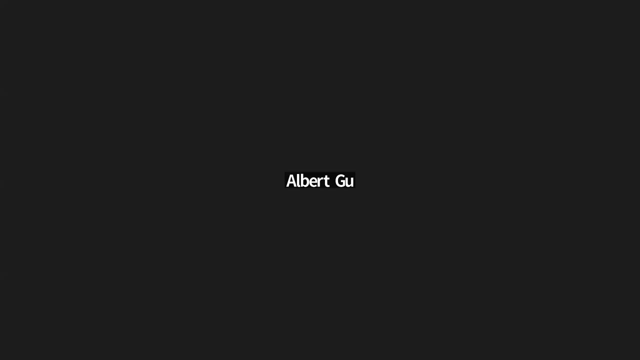 a number of benefits over other models just because, um, if you're in a setting where you need to like, if you're in a stateful setting where you need to be like updating your state as you go, such as, um i don't know, in like ro, robotics or something um, partially observed environments, uh, are like. 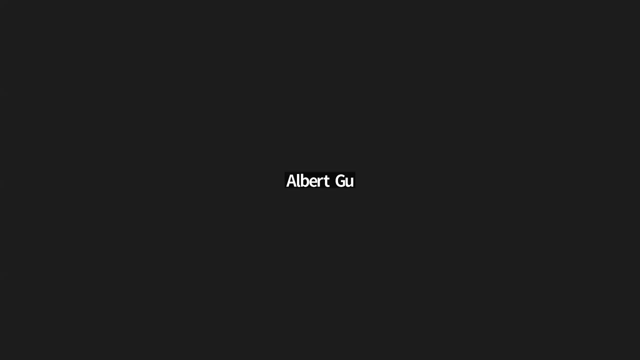 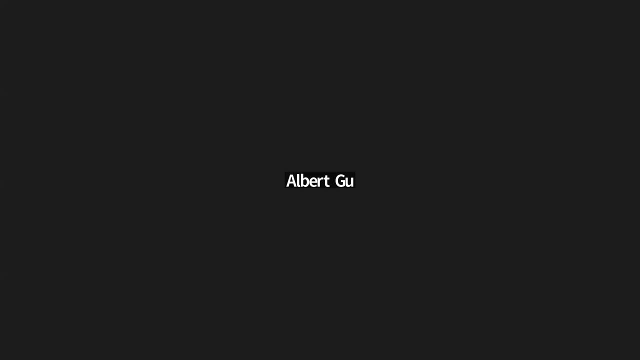 i do think of ssms and s4 essentially as probably like just the best version of an rnn that you can have um and lots of both, because of computational reasons and because of modeling reasons, like the vanishing gradients problem, the how do you get long context problem, um it empirically. 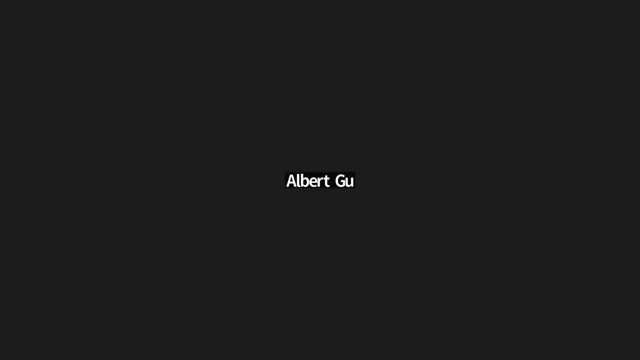 is pretty much just always performed better than like lstms or other things. um, i think there might be more. yeah, i, i, i can look at the zoom now. so i think, yeah, pc just uh gone through all the time. okay, great, okay, great. one more question, yeah, yeah, 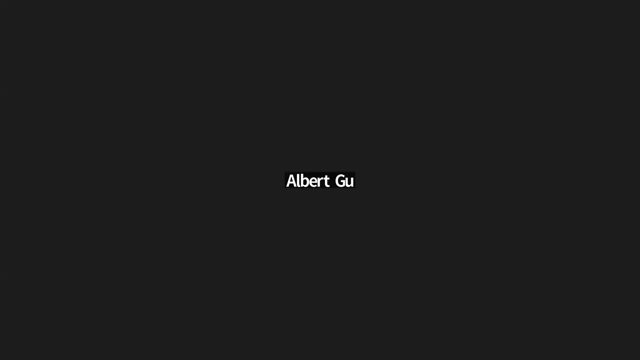 um, so this is, that's something that you can do, but you would have to, uh, view the model completely in recurrent form. so one way to look at this is that the convolutional view of ssms is tied to the fact that it's a time time invariant, or like, if you're uniformly sampling things, then you get the